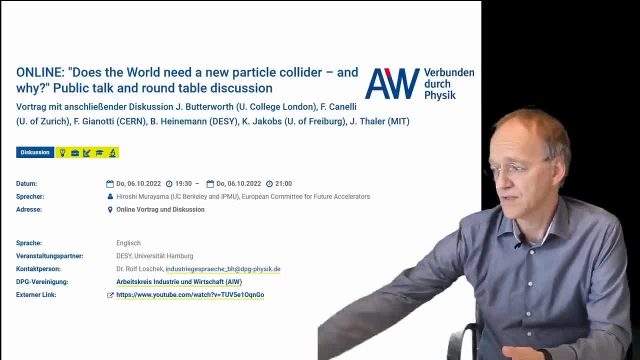 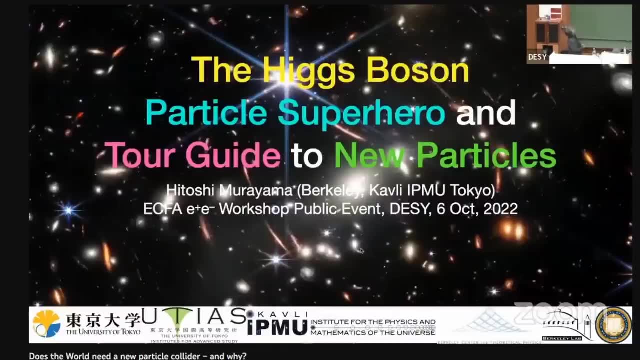 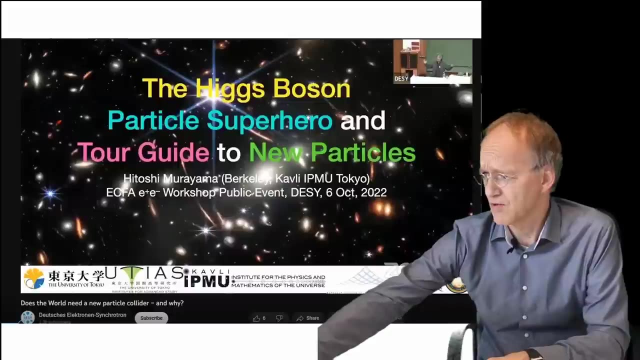 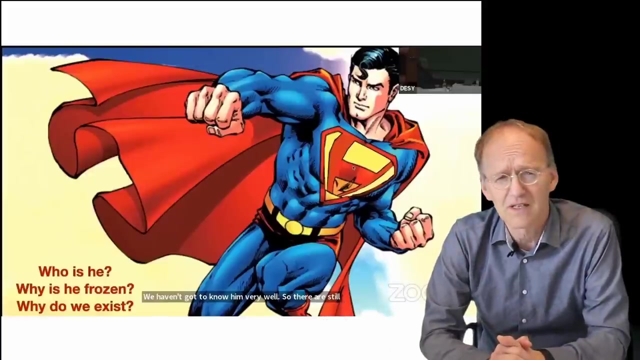 react to questions at the end. the talk is not online any longer, but i let you watch some of the highlights. my title today is the higgs boson particle superhero. to begin with, uh mayurama calls the higgs boson a superhero and superman, and this is one of his slides, and uh, well, i is it really? 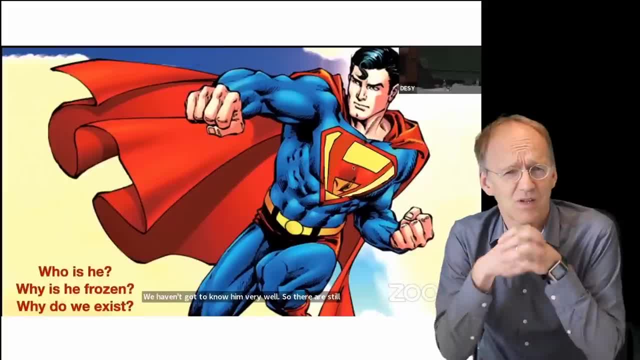 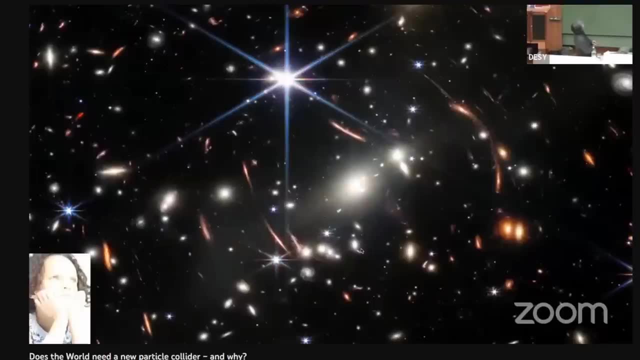 necessary that we resort to this intellectual level if you want to get interested the public about fundamental physics? i don't know, but now let's listen to what he said. so what physicists do is actually something very simple. we look at the night sky just like a little. 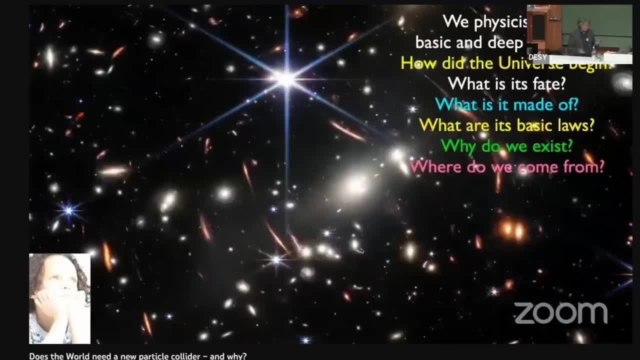 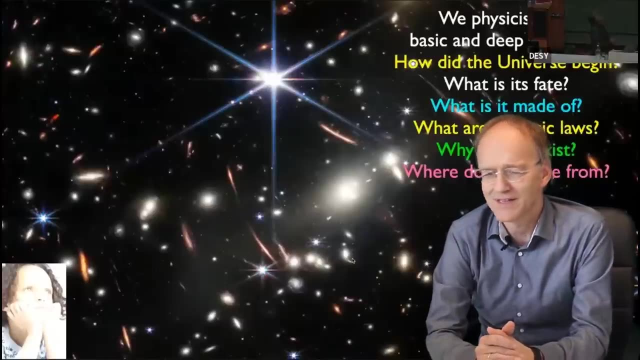 kid and start wondering some deep or simple questions like: how did the universe begin? what is its fate, what it's made of, what are its basic laws? why do we exist? where do we come from? well, none of these questions might be answered by a new collider or have. 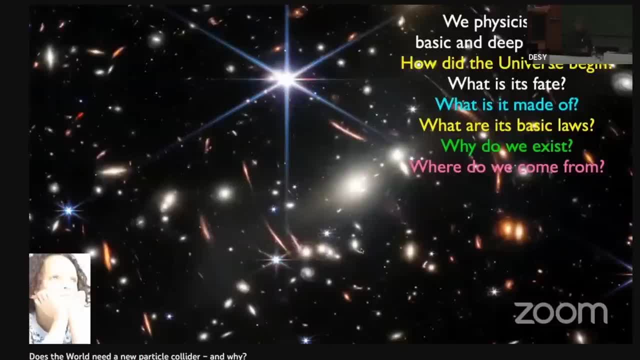 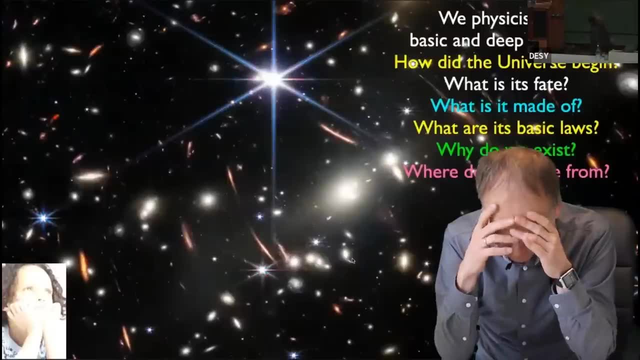 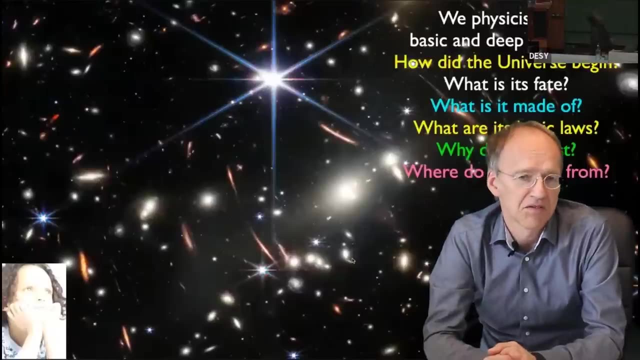 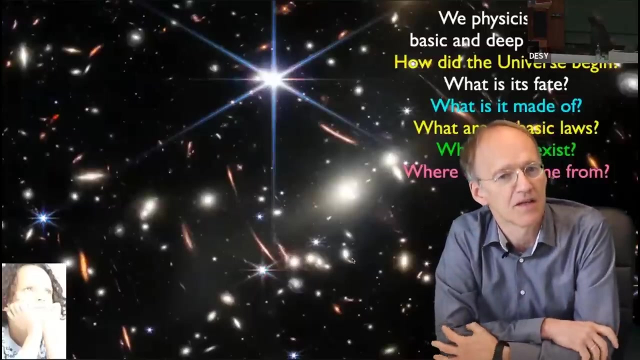 anything remotely to do with it. and the story today really has to do a lot with the question: why do we exist? well, humankind in 2022 didn't know why they exist. no, not, not at all, not because of physics results and not because of biology and evolution. and all this, no, no, no, no. but the new particle collider will. 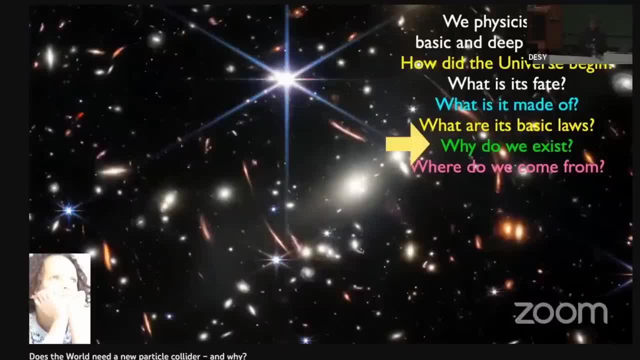 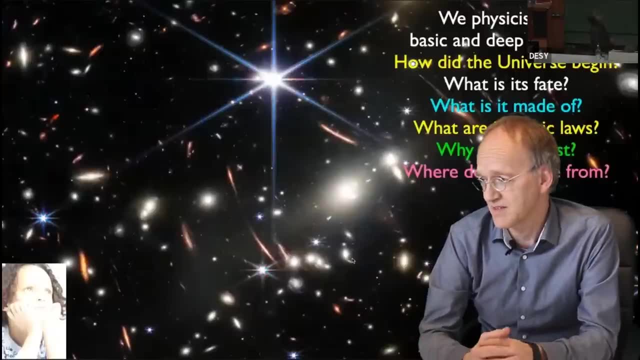 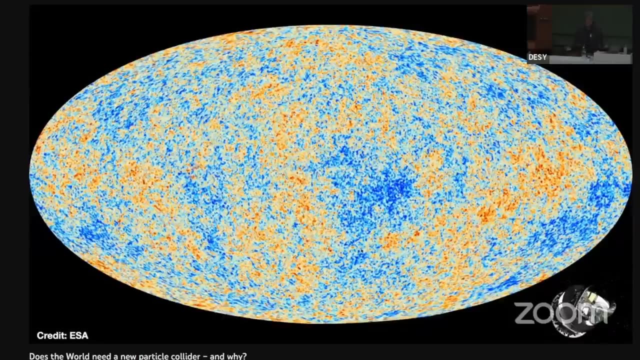 tell you, this kind of question used to be part of the philosophy, maybe. well, particle physicists are talking in a manner worse than the worst philosophers about this, but again, this is highly misleading. and this is the picture of the big man. you can actually see it in front of you. well, apart from this statement being nonsense, it's amazing. 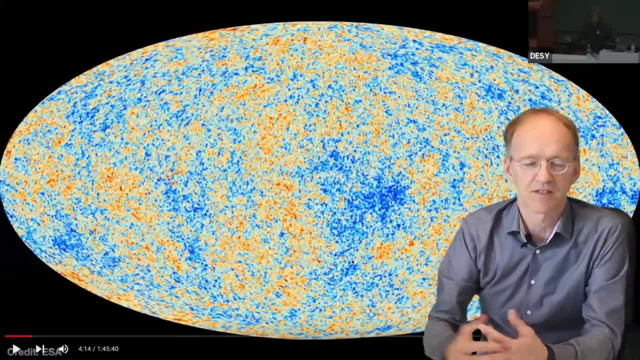 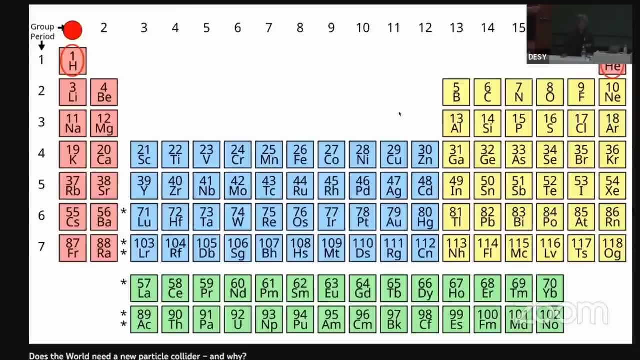 how brazenly these people take all kind of scientific results as if they had contributed to it. only hydrogen and helium were made in the big best. but for your body you need calcium, for your bone iron. for blood you need to breathe the oxygen where they came from. again he jump. 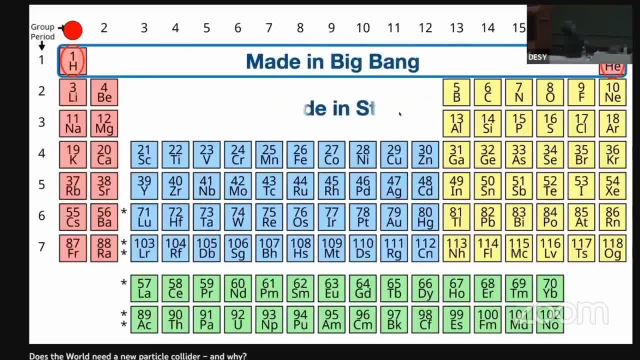 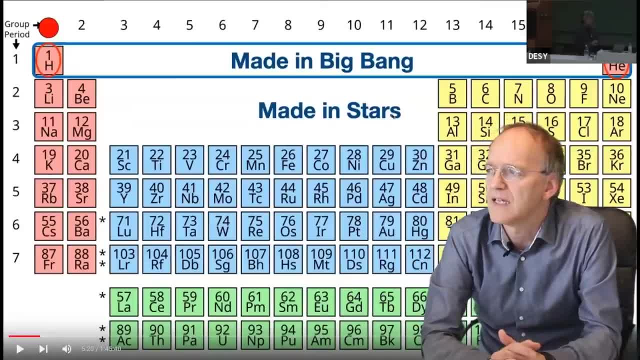 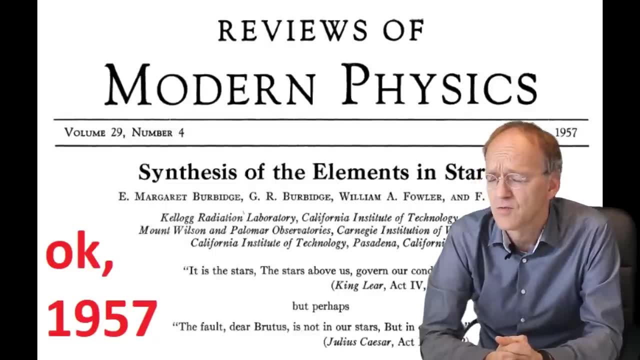 it turned out that they were actually made in stars. So this is something we have learned rather recently. This is something we have learned recently- I guess this is a result from 1952, the B2FH famous paper And again. 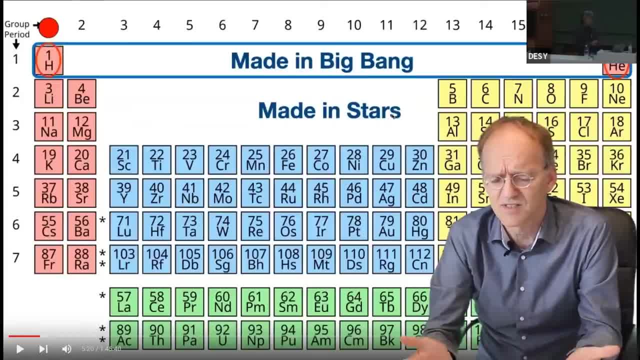 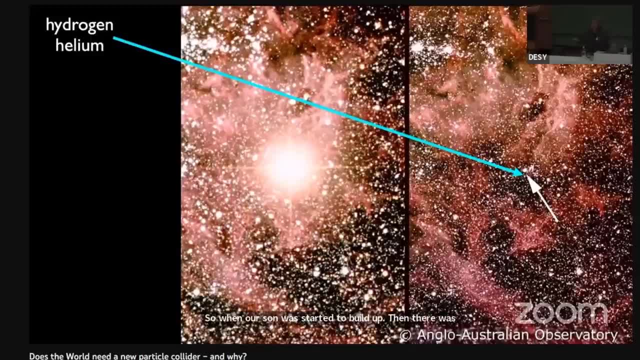 I mean, how dare you to assign this result to particle physics? It has nothing to do with it. Dust made up elements like oxygen and calcium and iron already in the dust that eventually hit each other, stuck with each other, developed to build a rock, and that's our planet. so that's how we 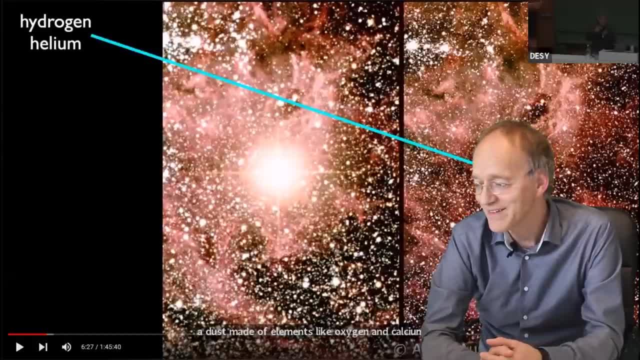 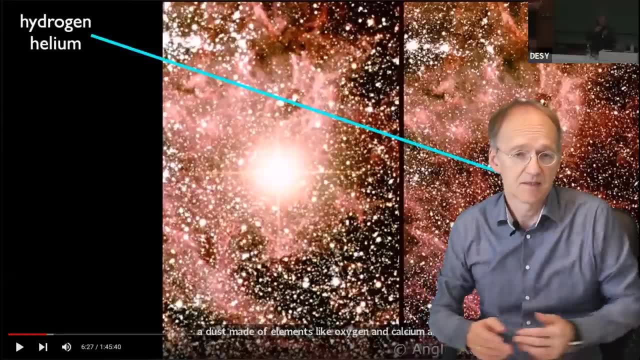 came to exist. Okay, quite a ridiculous statement, but again they're taking the results of astronomy and sell it if it was theirs. Interestingly, besides the Higgs, he does not mention a single result of particle physics of the last decades, probably not to remind the audience. 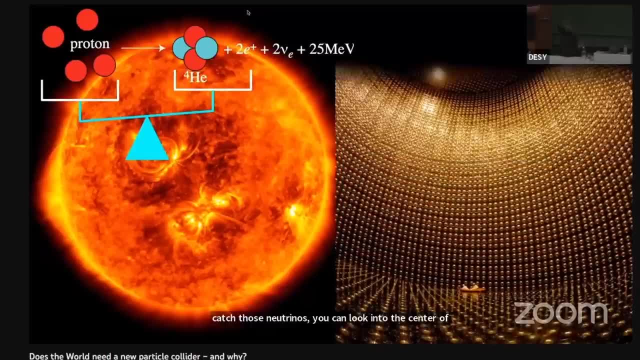 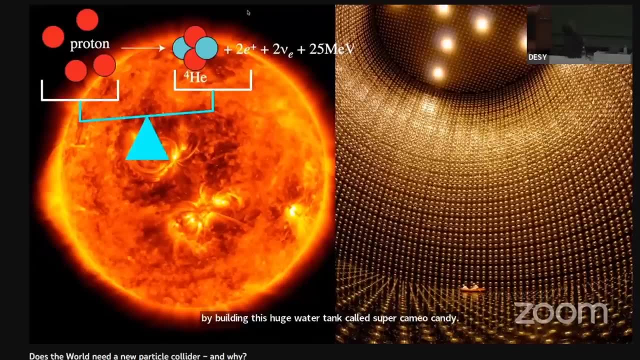 from its uselessness, And that's what my friends in Japan have done by building this huge water tank called Super-Kamiokande, and they even managed to take a picture of the center of the Sun, Completely misleading, and it has nothing to do with collider physics. 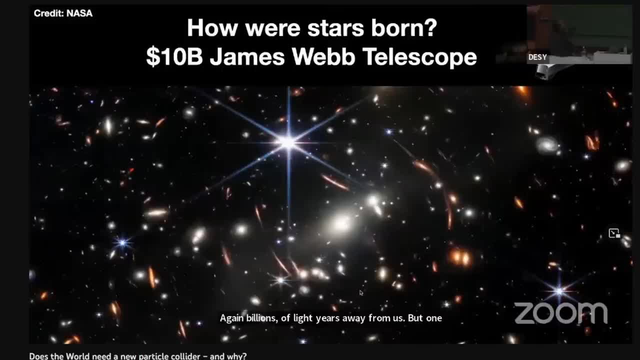 Sorry, But one thing you would notice right away is that there's some strange object in this picture. Galaxies are supposed to be round, maybe sometimes a little elliptical, but you don't expect to see something this much stretched out. But you see many of these things. This one is also very stretched out, that one. 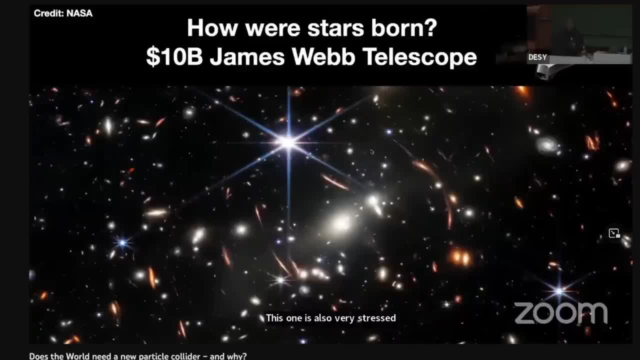 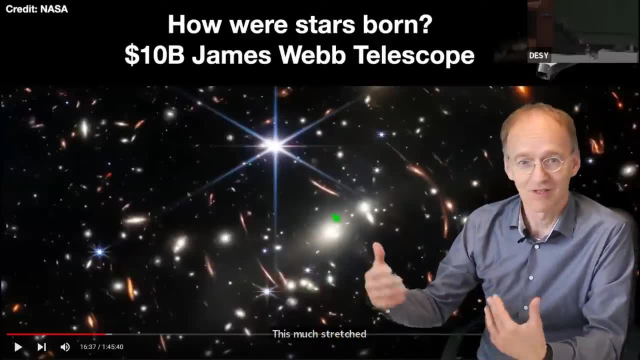 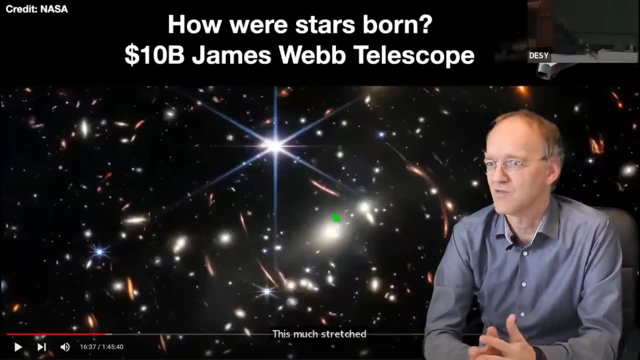 is two, that one is two. How could there be such strange shaped galaxies, Ridiculous? They grab a picture of the James Webb telescope, which is a real good science enterprise, and talk about gravitational lensing. I mean, gravitational lensing was discovered in 1979,. 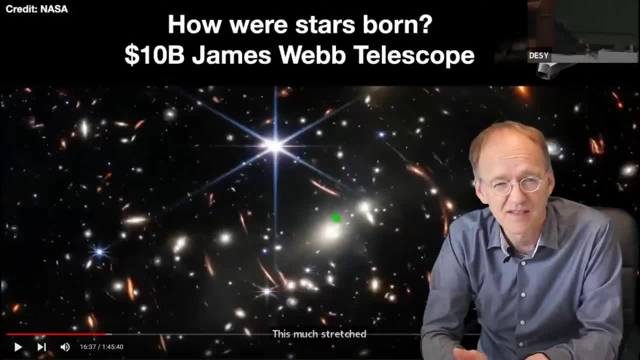 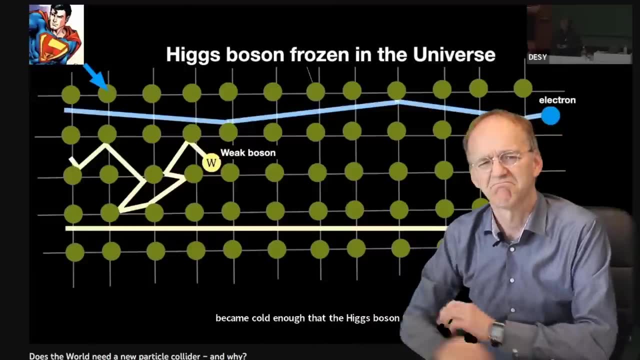 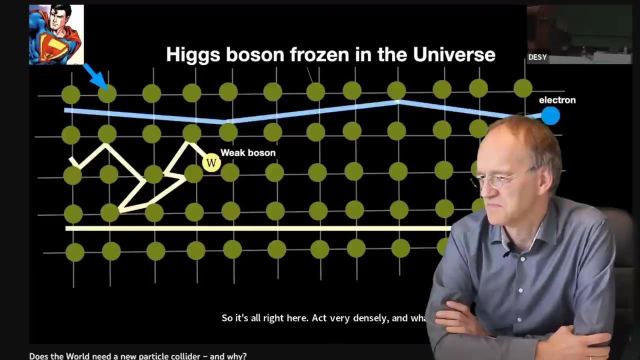 so what? That answers the question of our existence. Are you kidding me? The universe became cold enough that the Higgs boson froze into empty space, So it's all right here, packed very densely, And what's going on here is that when weak force wants to act on somebody, 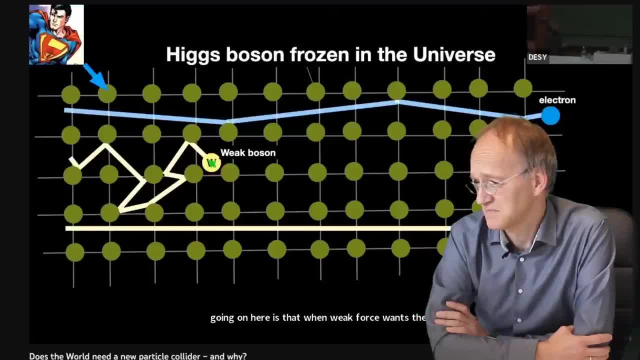 then it gets so much disturbed by this Higgs boson stuck in the universe today, and that's why it can't go very far. That's why stars would shine at exactly the right rate so that we can exist. This is also news to me. 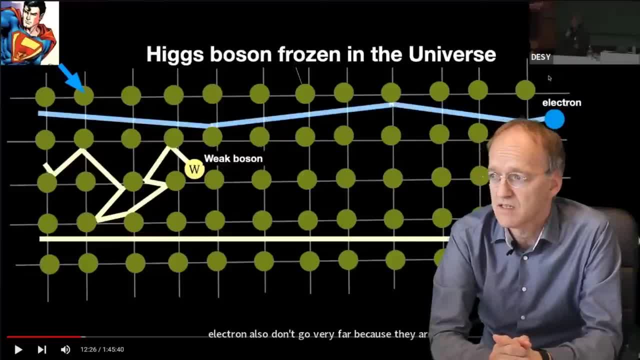 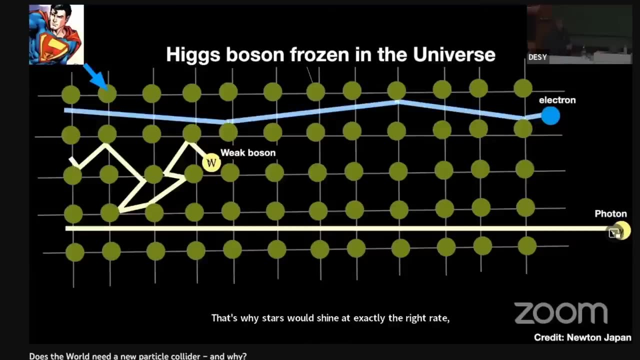 I mean not the discoverers of nuclear reactions in the sun, not the pioneers like Eddington or Jeans or whoever explained why stars shine. no, the Higgs boson does. That's really news to me. What it also means, though, is that the particles, like electrons, 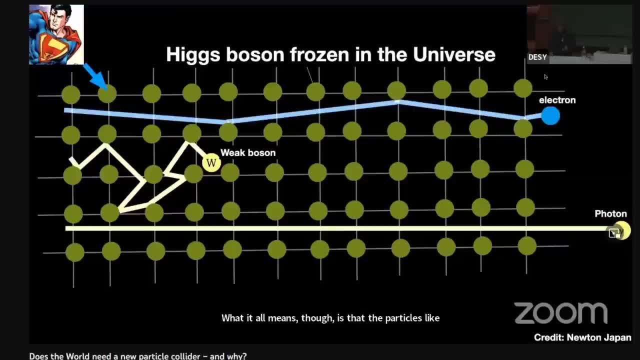 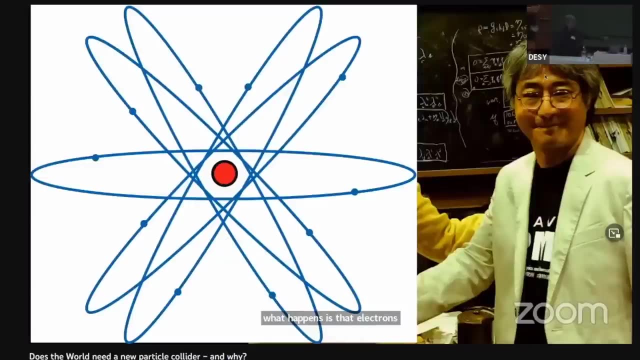 also don't go very far, because they are disturbed by the Higgs boson as well, which is the good thing, Because if this Higgs boson is not there, what happens is that electrons inside any atoms will start moving with the speed of light and instantly. 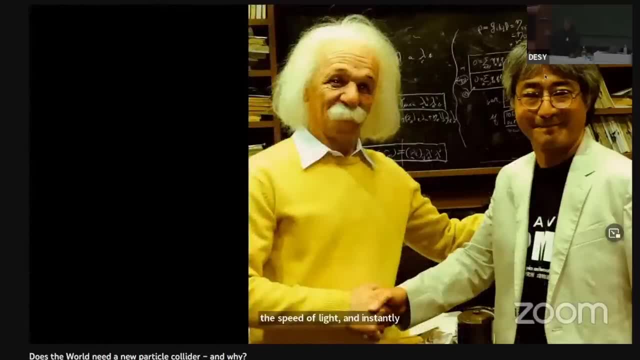 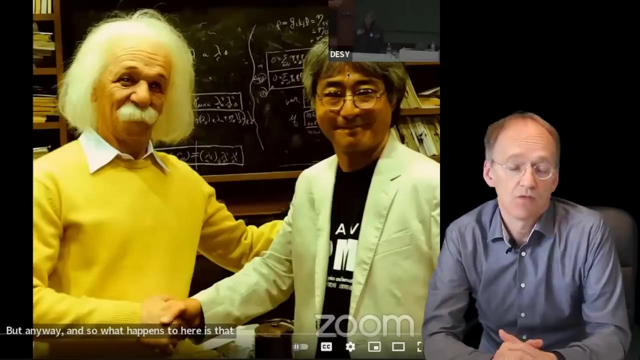 disappear, And you can see, I'm old enough to have a picture with Einstein in color, which is hard to believe, but anyway. And so what happens here is that we all evaporate in a nanosecond too. You would get evaporated in a nanosecond, yes. 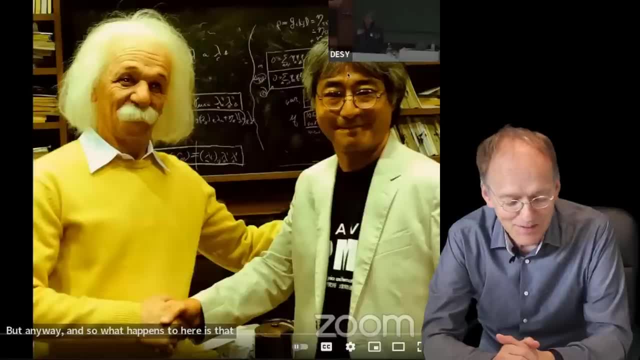 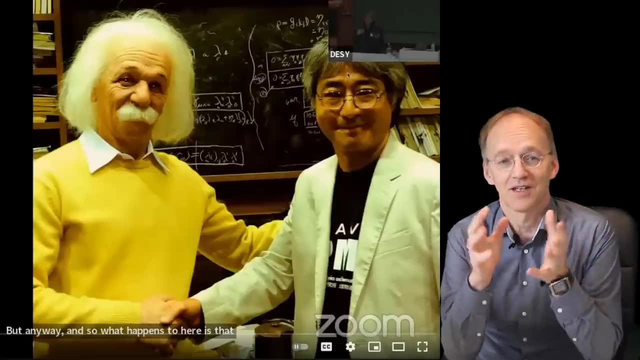 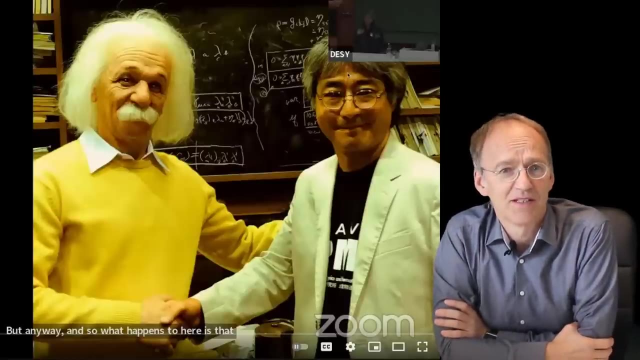 Of course, I mean, this is complete fantasy, but he talks to you as if the LHC had saved personally you from annihilation. And this superhero, Higgs boson, did all this. I mean what it actually did: it saved particle physics. 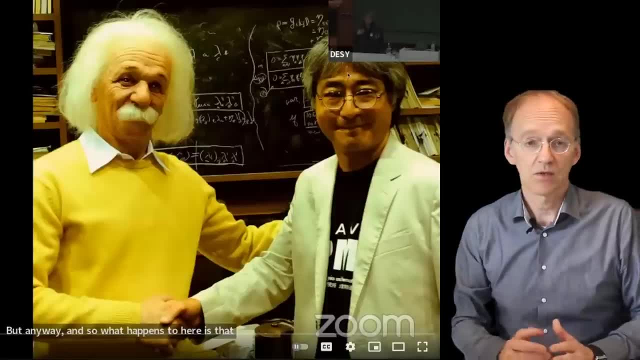 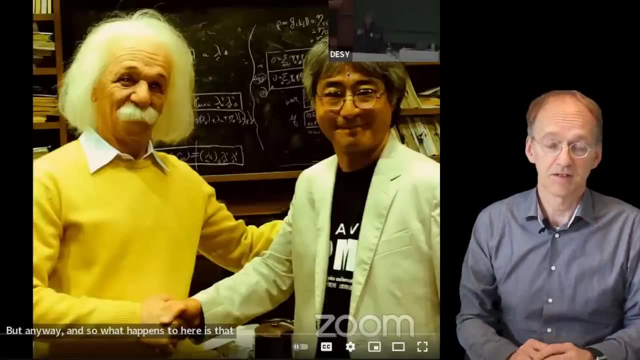 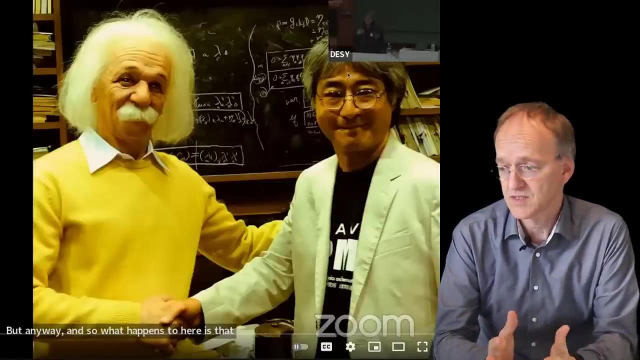 from getting their funding cut. So he continued to talk in this bold manner, as if the new collider would explain all these problems and solve all these interesting questions. Well, of course, all this pompous talking annoyed me quite a bit, and that's why I asked the question: why haven't these problems been? 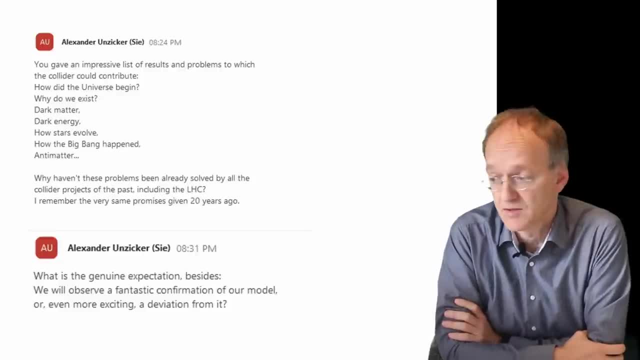 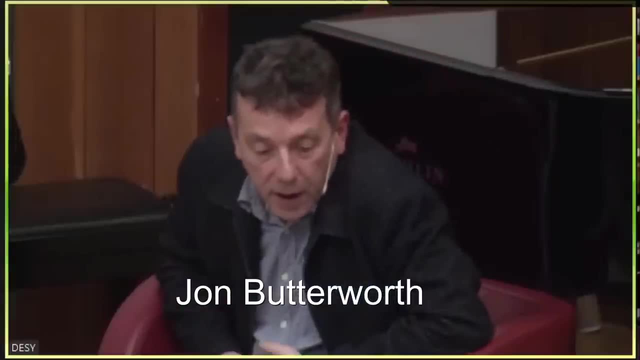 already solved by all the collider projects of the past, including the LHC. I remember the very same promises given 20 years ago. We have a question online which is referring back to the problems in Hitoshi's talk. Why haven't these open questions already been solved by the collider projects of the past, including 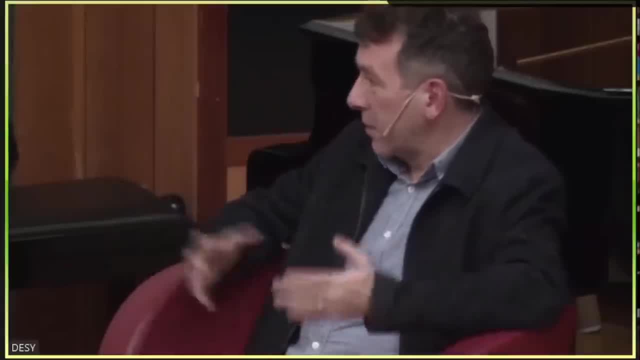 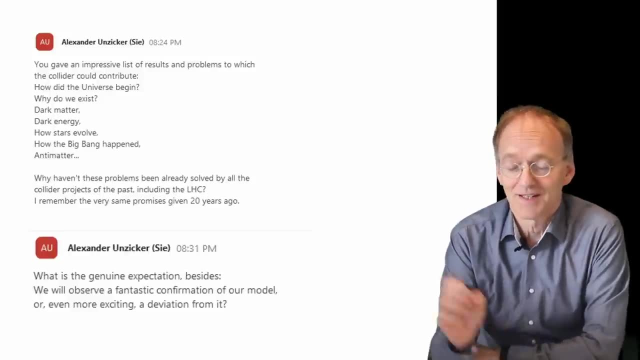 the LHC. The question says: you know, I remember hearing some of these questions being asked 20 years ago and they're still not answered. So why is that? What's the case? And actually Butterworth rephrases the question a little bit If you listen carefully. he says: 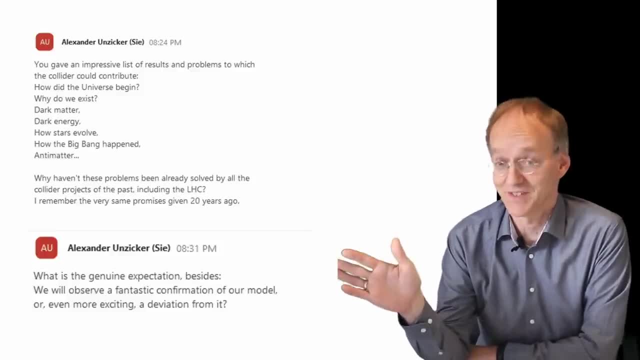 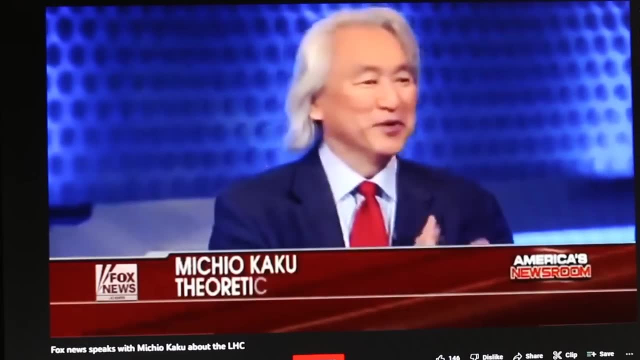 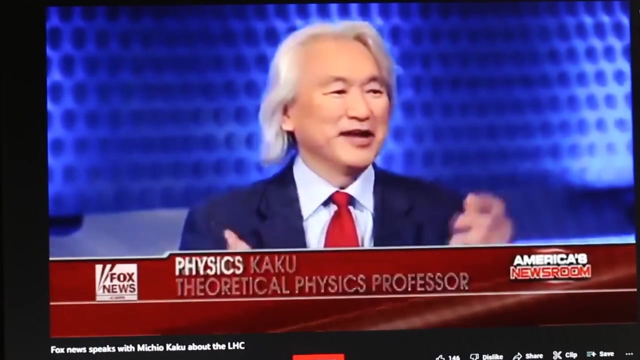 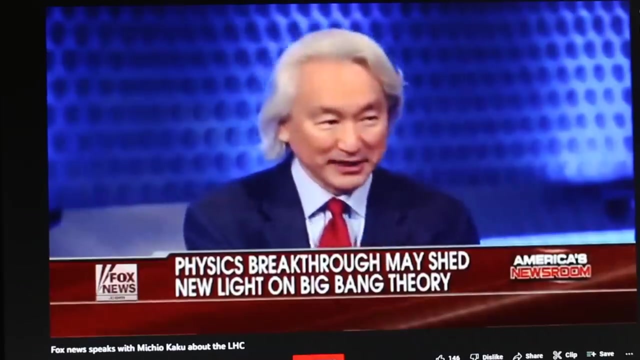 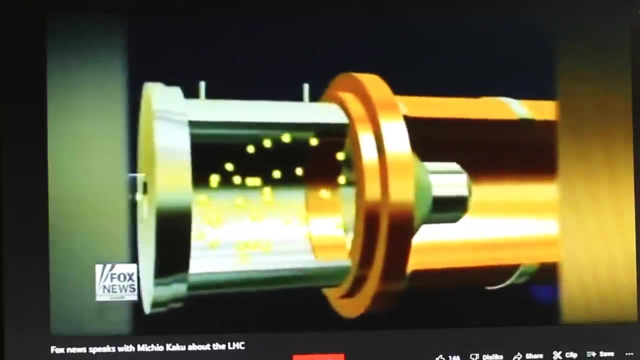 questions, not promises, but actually these were promises. Listen to another theoretical physicist, Michio Kaku, 12 years ago: Genesis, chapter 1,, verse 1, and also maybe even answer eternal questions like time: Is time travel possible? Are there other? 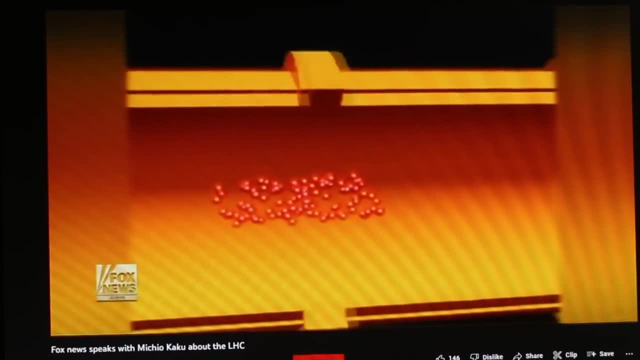 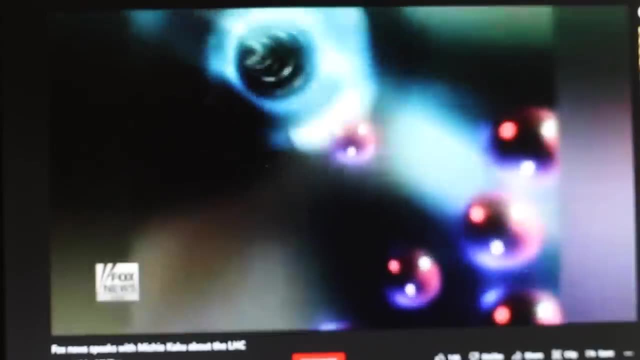 dimensions? Are there parallel universes? We can get hints, glimmers of these cosmic questions with this machine. So you think we can figure out what happened before the Big Bang. You think we can figure out whether or not time travel is possible Because of what they're doing on the French-Swiss border. 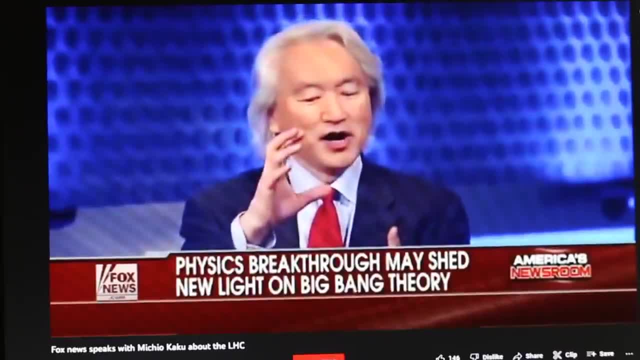 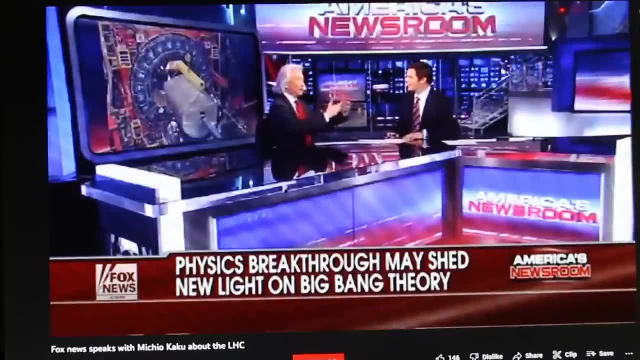 That's right. And maybe our universe is a bubble of some sort and there are other bubbles out there, Other expanding and contracting bubbles. And what would these other bubbles mean to you? These are other universes where perhaps there could be other laws of physics. 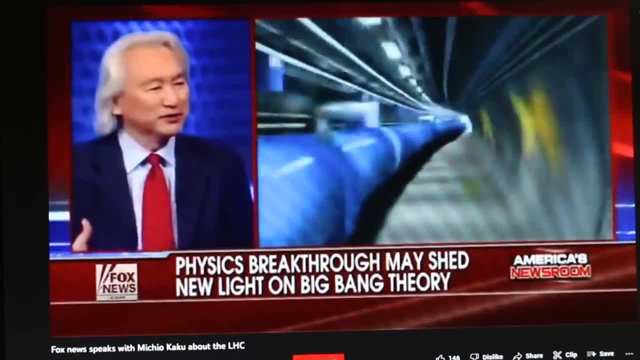 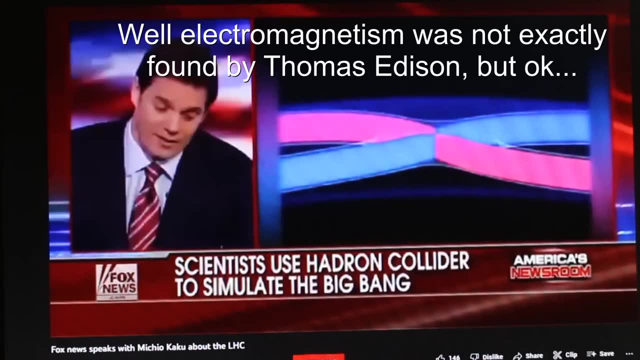 I mean this is huge Really. This is greater than the Copernican Revolution. That's what the Large Hadron Collider can do. So you're putting this up there with Sir Isaac Newton and gravity. You're putting that up there with Thomas Edison and electromagnetism. That's right. 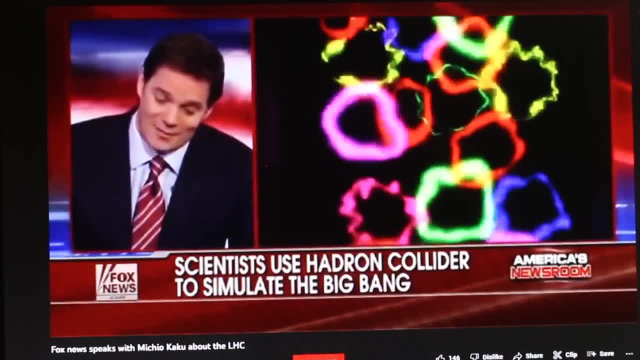 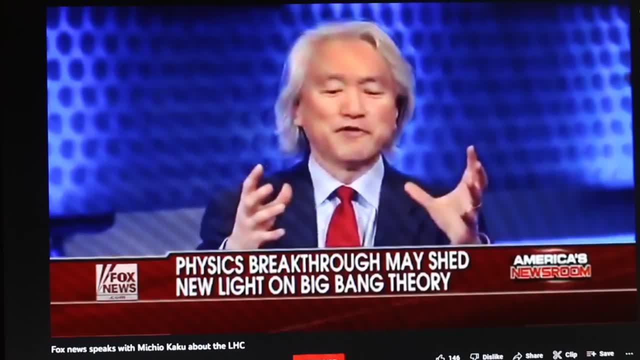 You're putting that up there with Albert Einstein and E equals mc squared was what? the nuclear power- That's what you're writing about today in the Wall Street Journal- Is that significant. It's that big. By unifying all the forces of nature- There are four forces that make the world- 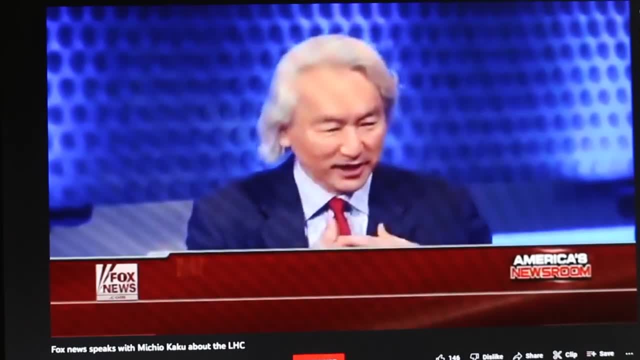 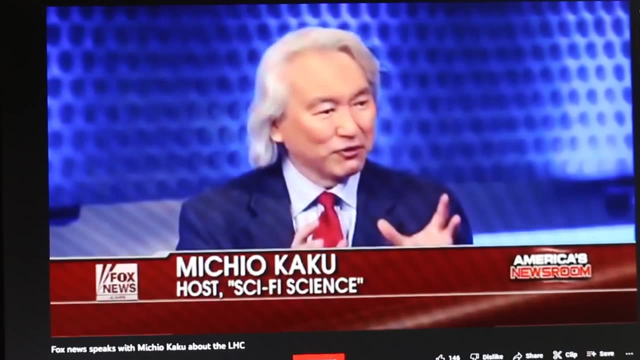 move. Each time a force was unraveled, it unleashed the Industrial Revolution, the Electric Revolution and now the Nuclear Revolution. And now we have a super force, A super force that we're going to try to unravel, which created the universe. Yeah, no comment so far. 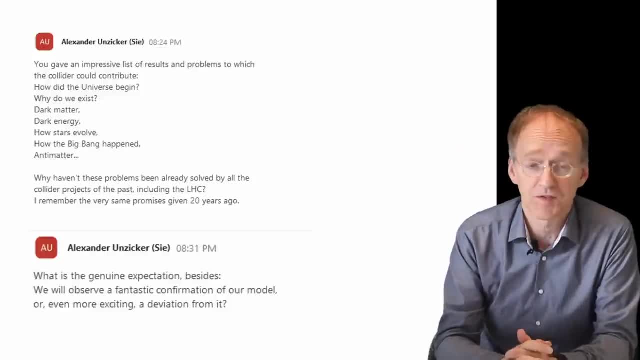 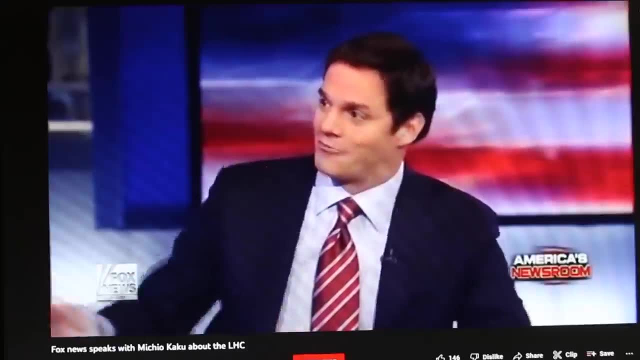 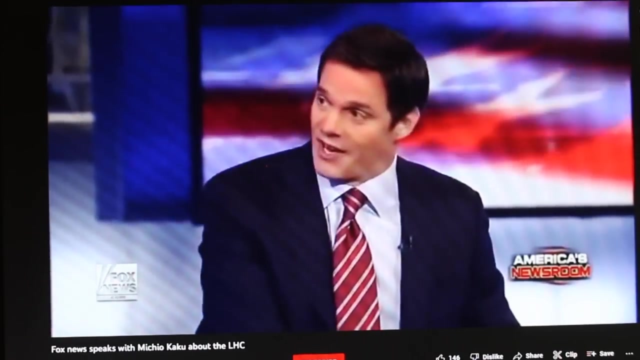 Kaku is another Japanese theoretical physicist, in the thinking tradition that you become an Einstein once you have white, unkempt hair. Physics professors who are conducting these experiments in Europe. it could have been happening here at home And you're suggesting there's a bit of a brain drain from the United States. 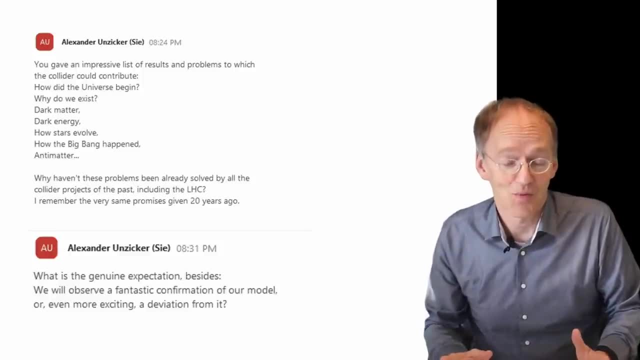 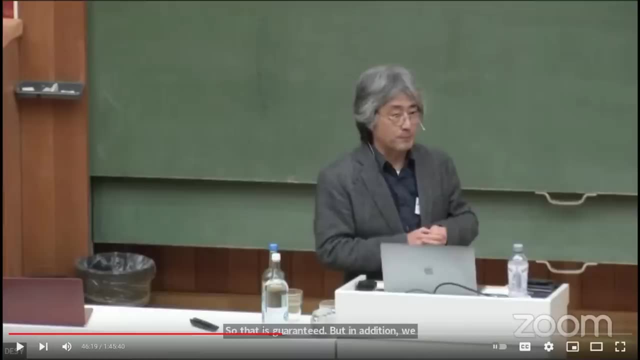 I'm glad that we avoided that kind of brain drain into Europe. but listen now what Majorama has to say. Well, at least for the Higgs boson, we basically just met him. It was discovered ten years ago. That's a very brief. 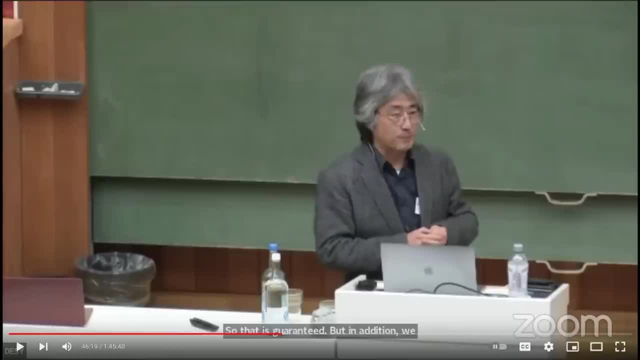 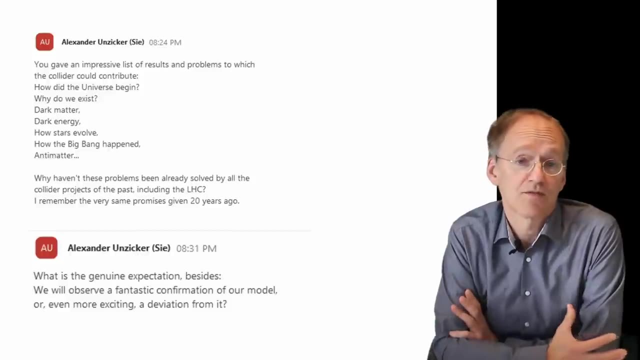 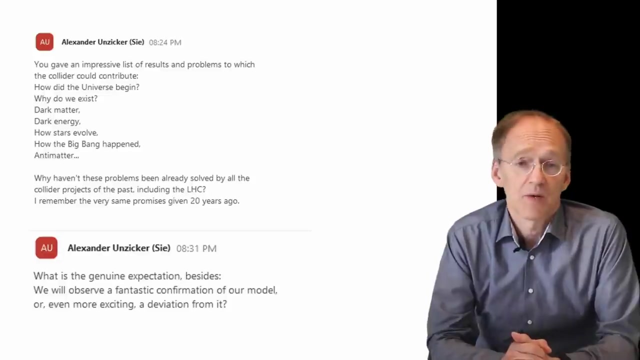 period in the history of science. So there's still a lot we haven't understood about this new superhero, Or we just have discovered the superhero, So we need to study more of it and we need to talk to him and we get more information. By the way, I added this question: What is the? 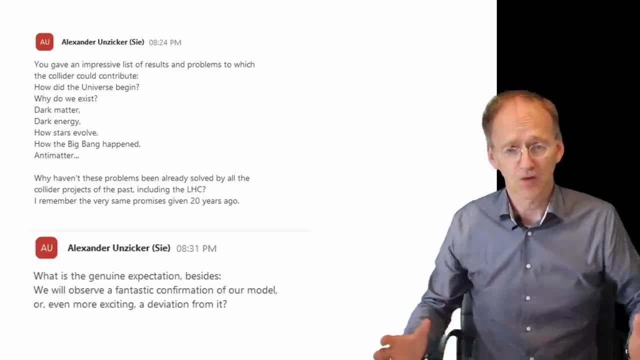 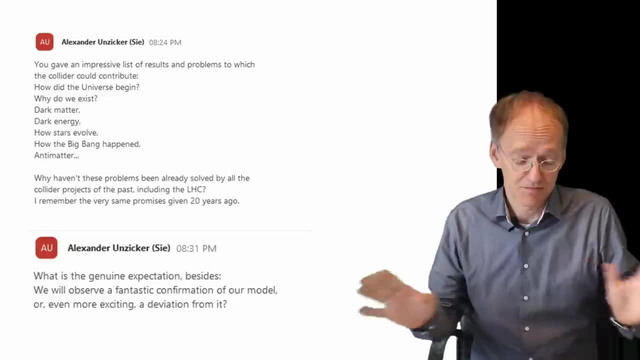 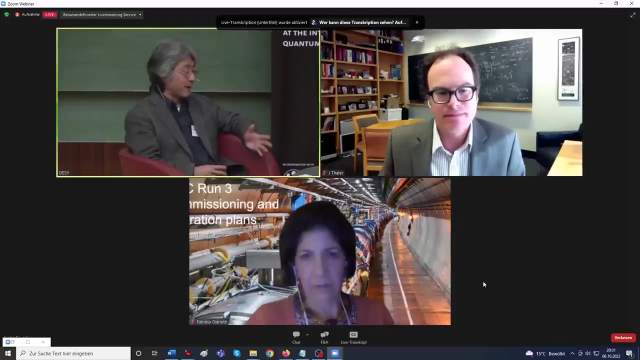 genuine expectation. Besides, we will observe fantastic confirmation of our model or, even more exciting, a deviation from it, But that's obviously. this was too hard, though Butterworth did not ask the question On the other questions, like dark matter and antimatter, if we were lucky. 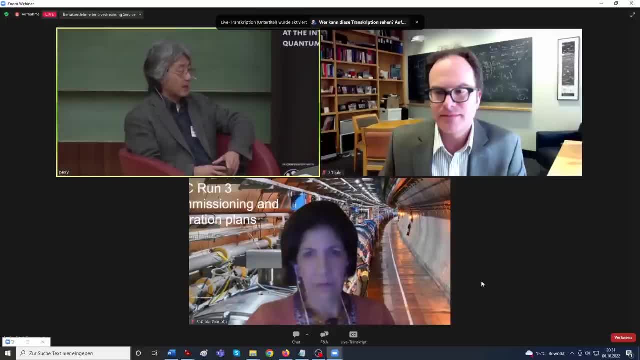 we might have seen some glimpse of answers in past experiments, but nature wasn't so generous to us, So they are still waiting to be discovered and understood. so we have to keep trying, And in this case, there's no guarantee that the next generation of 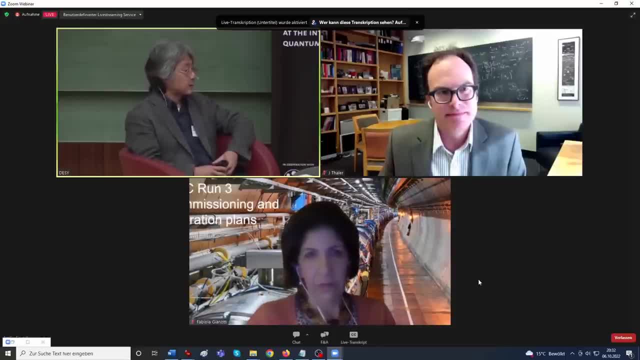 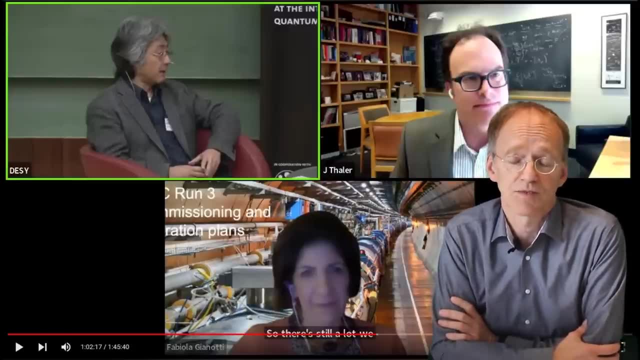 colliders actually answers those questions, but at least I see a good chance. Yeah, and of course we have a good chance to see the undiscovered particles in the next collider experiment. of course Let's also listen what the others have to say. 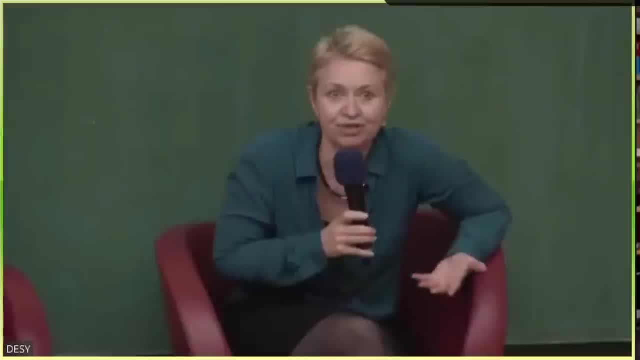 The Higgs could decay to dark matter and when it was discovered, basically it was possible that nearly all of them we could only. I mean the way the Higgs boson was observed was in a very, very rare decay. What A rare decay. The Higgs was discovered. 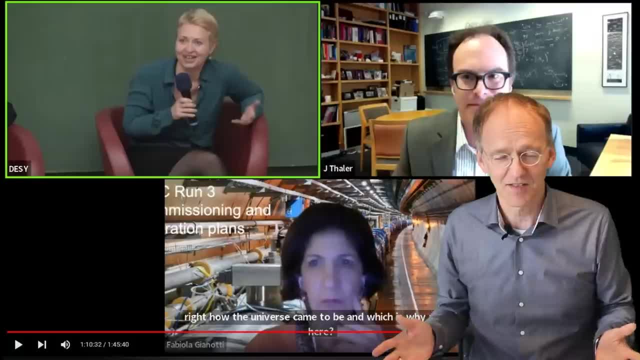 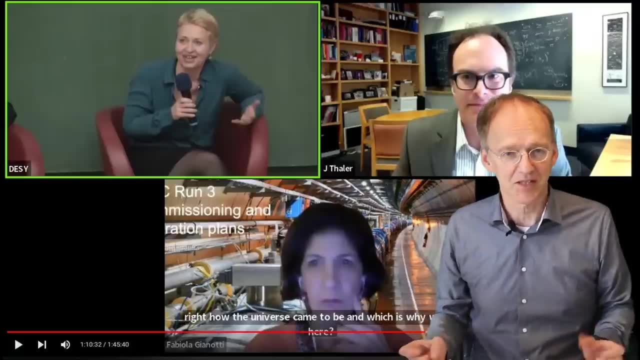 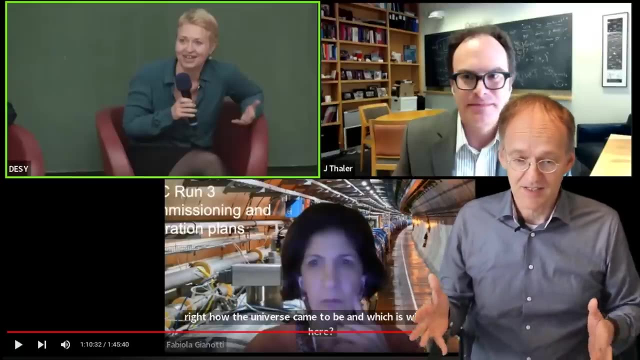 in the two-photon channel, which is the most dirty channel, so to speak, because literally every particle and antiparticle decays into two photons. There is nothing special, And of course the reasoning was why it was so hilarious that they argued that the Higgs has been discovered. because they argued that. 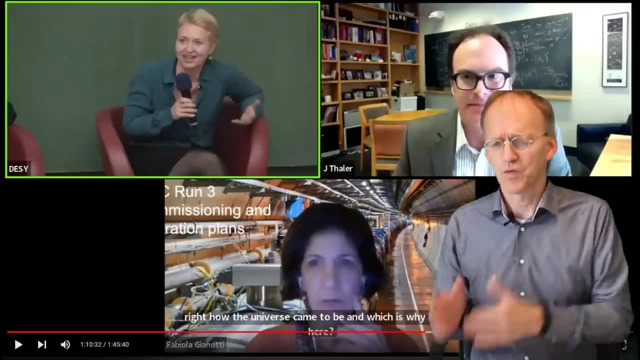 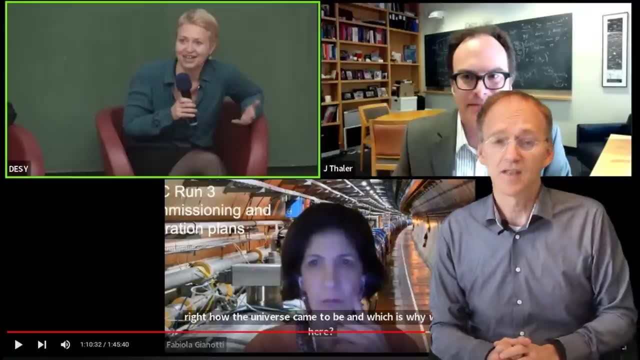 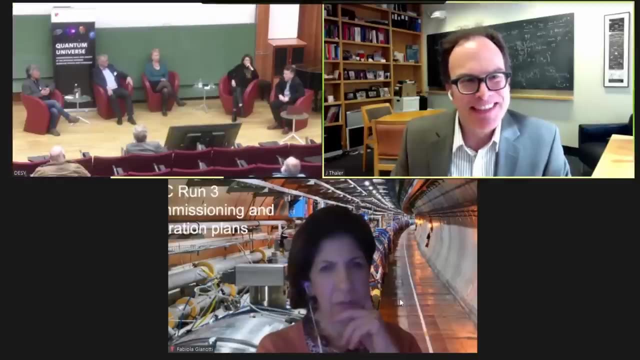 oh, we perfectly know which kind of particles decay into two photons, and there are billions of decays, and one in one hundred billion decays is not explainable by our model. So this must have been the Higgs boson decay. Can I answer that question? Yeah, go ahead, Jesse. 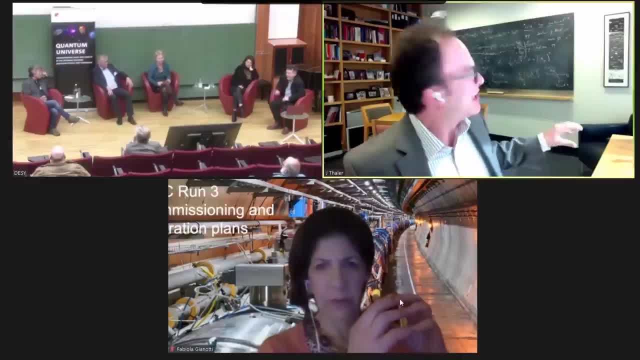 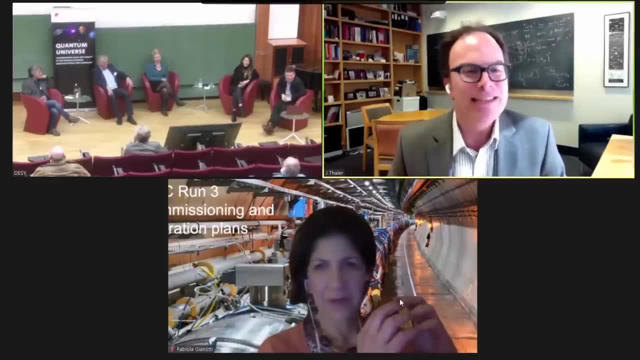 Well, it's fun for me to answer that question because I was just explaining it on the blackboard over here. Maybe you can't really tell. So you know, I'm a professor at MIT and I have students who come into my office who ask: you know, why is it that I should focus? 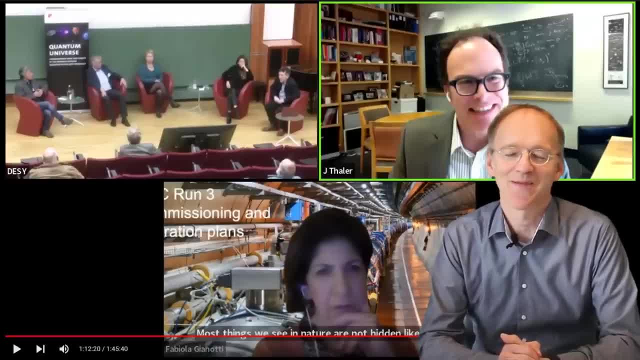 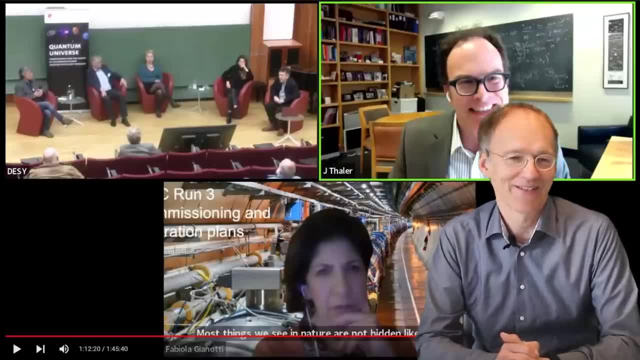 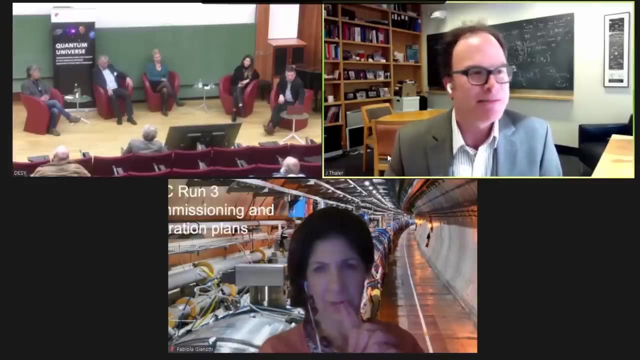 on doing calculations. I like so much explaining because I'm a professor at MIT and I'm so smart that the students come into my office and I explain to them all these difficult calculations And you can estimate how much precision you need in order to answer some of the questions. 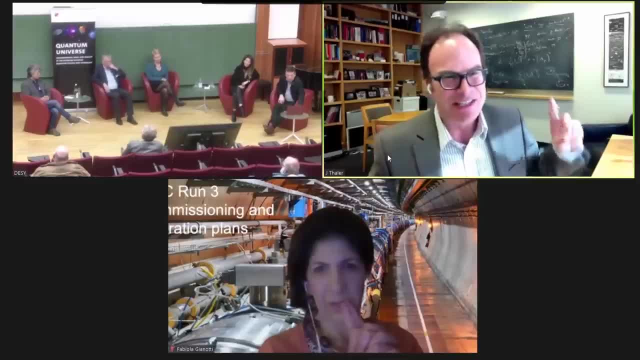 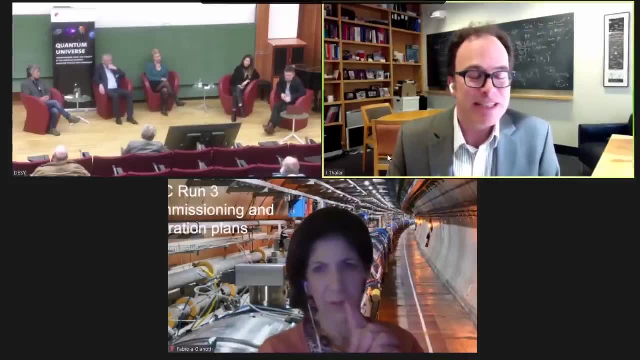 that Hitoshi was talking about And this back of the envelope thing that's on this board here was explaining why if you don't do better than 10% accuracy, then you really can't address these deep, fundamental questions. Oh, you're saying that you need 10% accuracy? What a 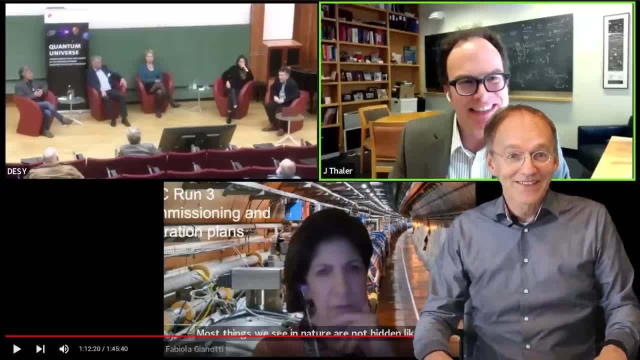 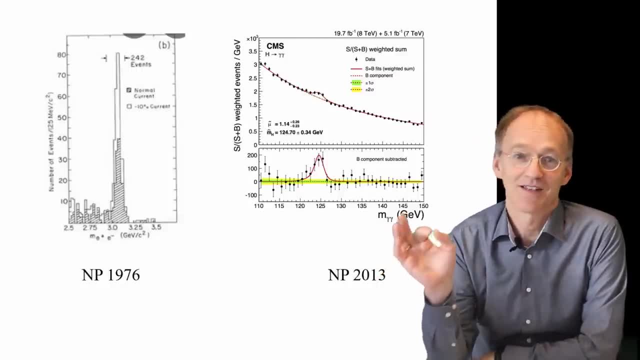 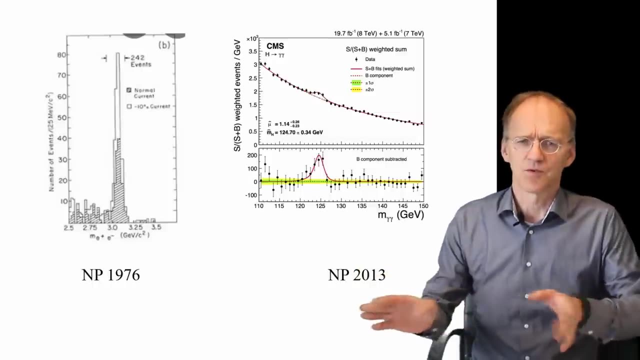 spectacular insight. I can't believe it. 10%. I tell you something: There was a time when particle physicists had fairly precise results, such as the Nobel Prize in 1976 for Ting and Richter. Not that I won't endorse that. 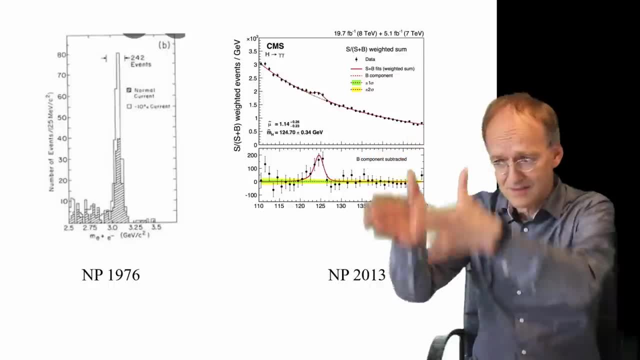 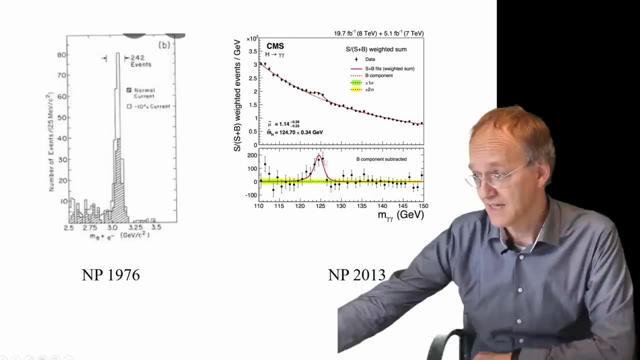 this is something significant, but at least it's some decent curve here, And if you look at the Higgs discovery, it's a very, very pure accuracy- On the other hand, around 6%. and now you're saying that the next collider will only 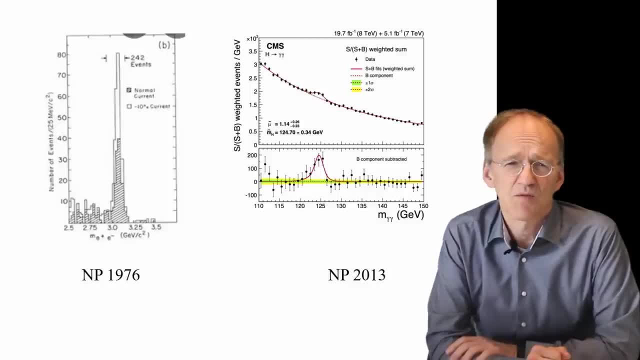 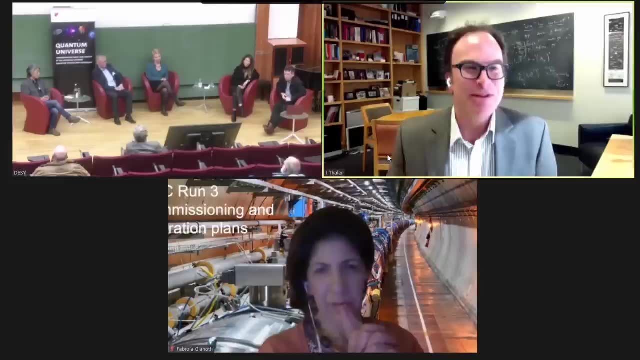 have 10% accuracy, That means you are free to interpret any kind of fantasy particle into such an experimental mess. if it's only 10%, I would love for it to be different. I would love for big ideas to have big manifestations. No comment so far. 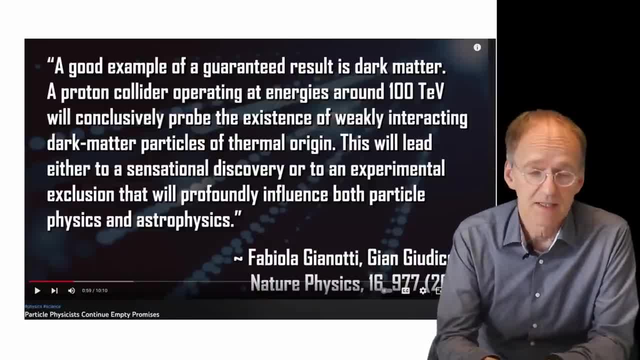 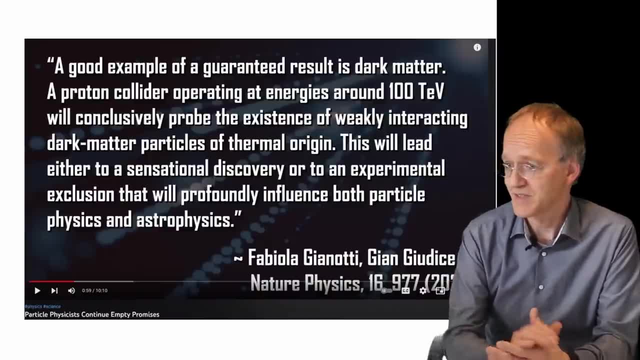 For my next question, I'll give it a little bit of context, because recently Sabine Hossenfelder had exposed the empty premises of particle physicists in a very nice video, And here is one slide with a quote of Gianotti. A good example of a guaranteed result is dark. 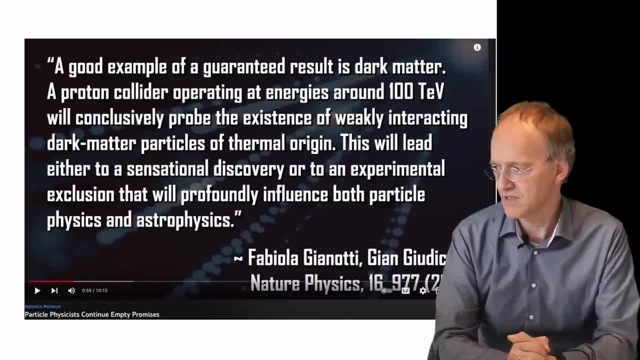 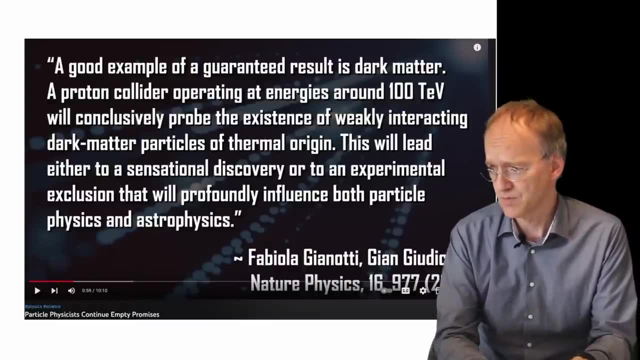 matter. A proton collider operating at energies around 100 tV will conclusively probe the existence of weakly interacting dark matter particles of thermal origin. This will lead either to a sensational discovery or to an experimental exclusion that will profoundly influence both particle physics and astrophysics. 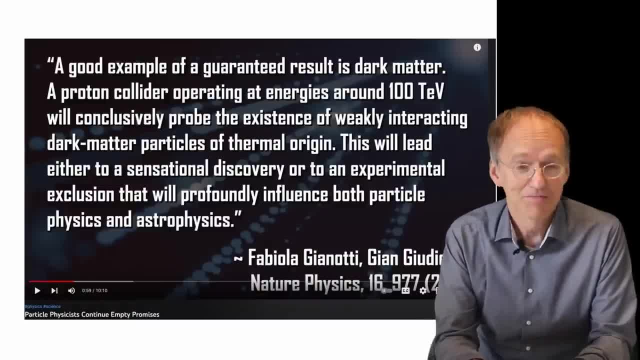 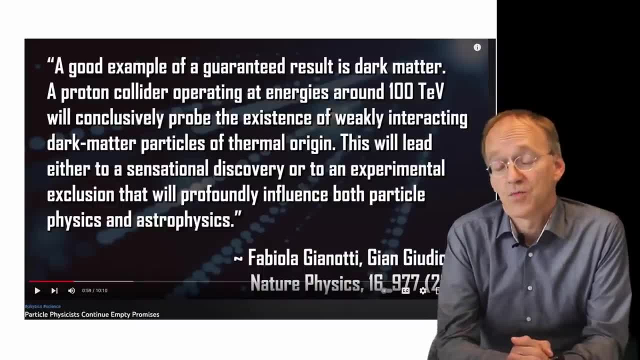 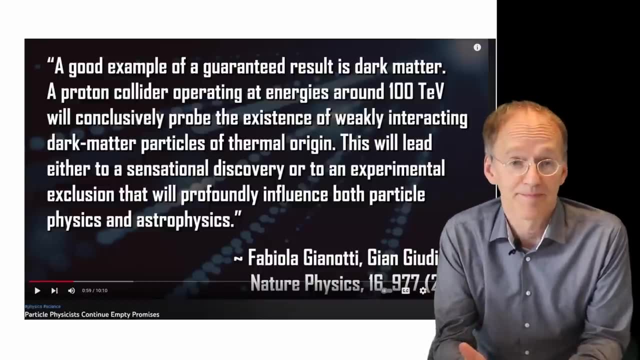 And Hossenfelder commented: no, the most likely outcome is that particle physicists will swap their current theories for new theories according to which the supposed particles are still heavier than expected, and then they will tell you they need a new collider to find them. 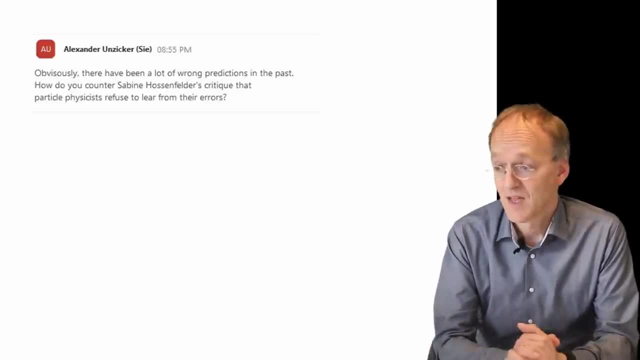 So my question was referring to this critique. obviously there have been a lot of wrong predictions in the past. How do you counter Sabine Hossenfelder's critique that particle physicists refuse to learn from their errors? Back to this business of new. 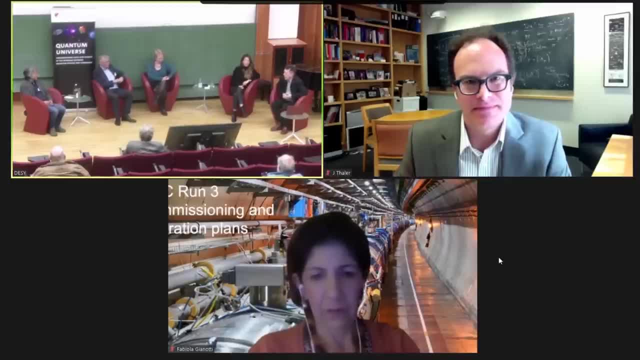 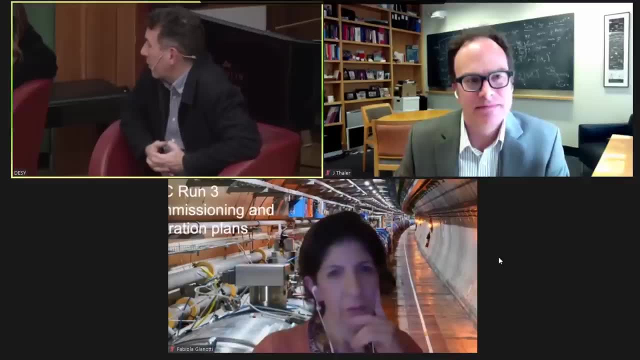 particles, though, We've had, and just to elaborate on it a little bit more, we've had. every time there's a new collider, the theorists will tell us: we're going to find all these new particles. The only one they've really been right about has been the Higgs, which is part of the 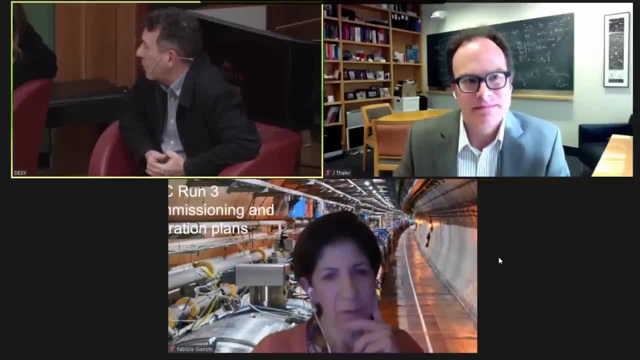 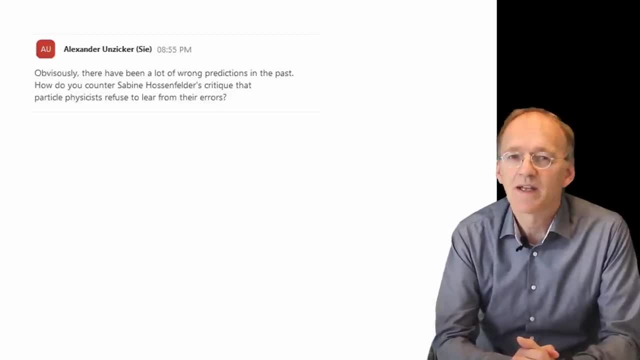 standard model. So are we flogging a dead horse here? Are we refusing to learn from our mistake? Butterworth did not mention Hossenfelder, but it seems that she understood that someone had exposed her empty parameters and she is hit. Look, No, no, no, no, no. 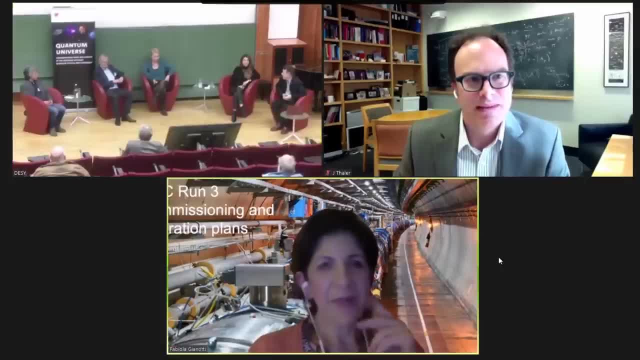 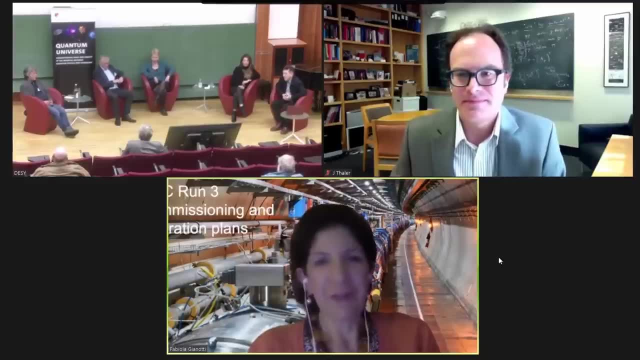 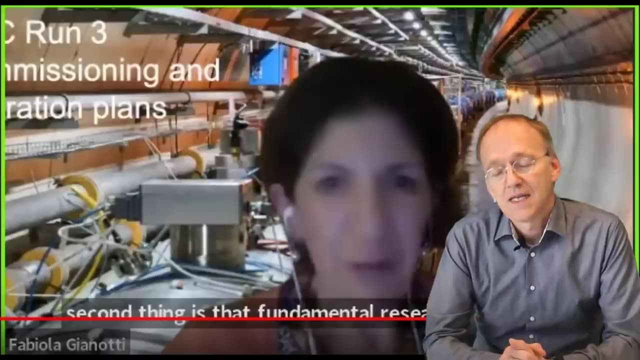 You can't say this, Can I, John? sorry, can I say something here? So I mean, of course, when you discover a new particle, of course this is a big satisfaction, it's a glamorous thing. you get the headlines of the newspaper. Yeah, the headlines. 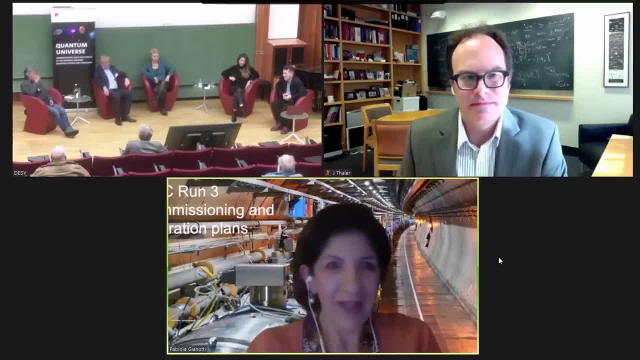 are important. Take a machine like a collider, like LEC, and Yutoshi mentioned it in his talk: LEC did not discover any new particle And it's hardly a machine, an accelerator, a collider that has really had such a profound. 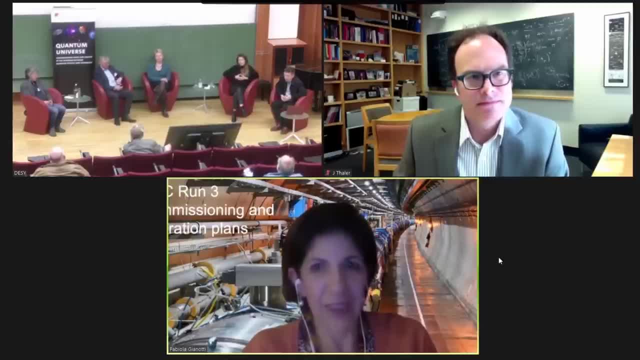 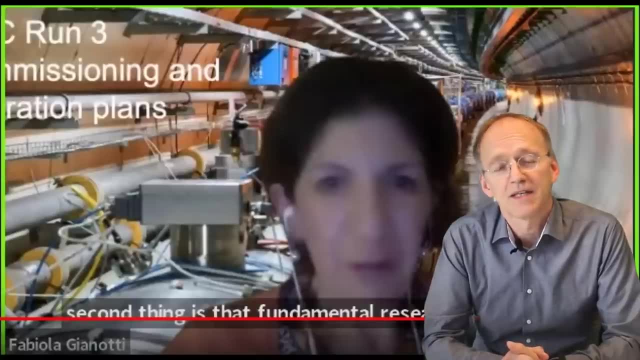 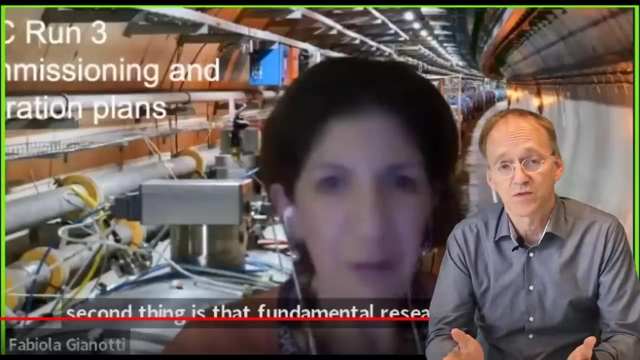 impact on our understanding of fundamental physics. It has put the standard model on solid experimental grounds. To put the standard model on solid grounds, whatever that means. What we want to do is to improve our knowledge is to make a step forward. My next question was rather 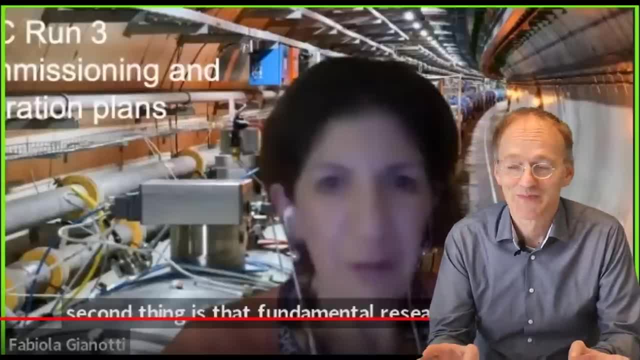 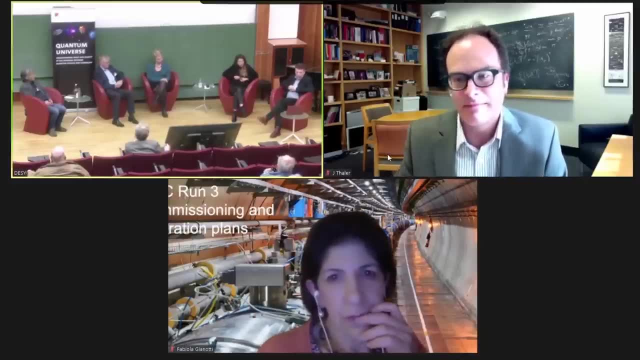 a mockery than a question, but everyone agreed it was a good question. There was one question which actually was explicitly addressed to Fabiola, in fact, which was: if the standard model is on solid ground, why is everyone excited about deviations from it? It's a good question. 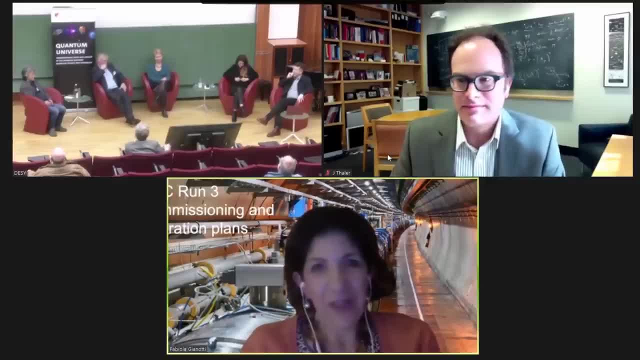 You start, Fabiola. Yeah, okay, so simply because the standard model cannot explain everything we see and everything we have understood. So Yutoshi was mentioning dark matter. we don't understand dark matter. there is no single particle in the standard model that has. 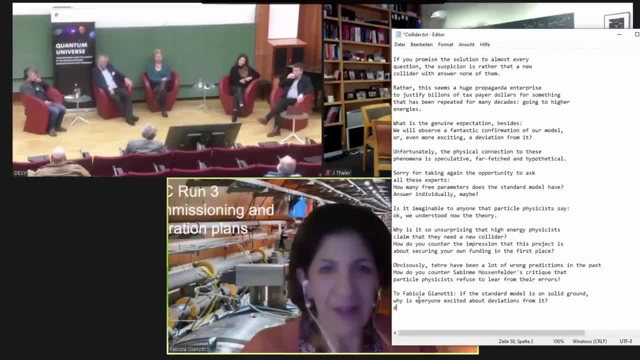 all the good properties for dark matter. We don't understand dark energy. we don't understand the matter-antimatter asymmetry. So the standard model works very well. its predictions are very well demonstrated. all the particles predicted by the standard model have been discovered. 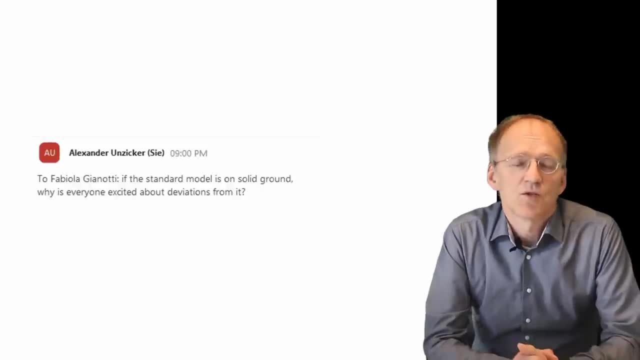 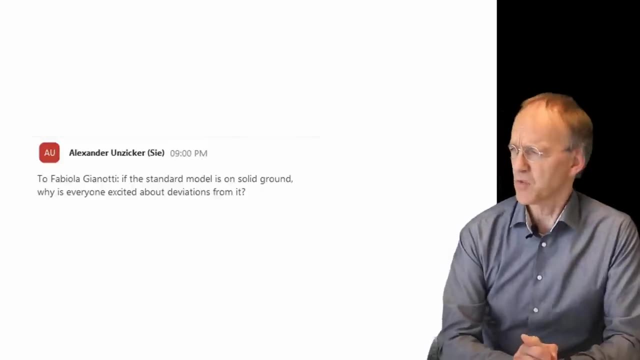 but it's not a complete theory. Yeah, this is the usual Orwellian doublespeak I really don't understand. in particle physics They say: oh, the standard model is so fantastic, tested, it's on solid ground, it predicts everything and wonderful. 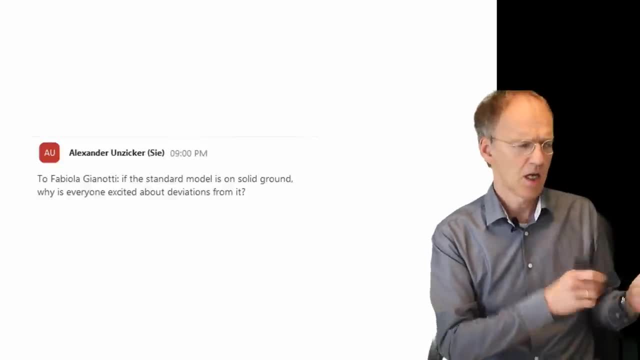 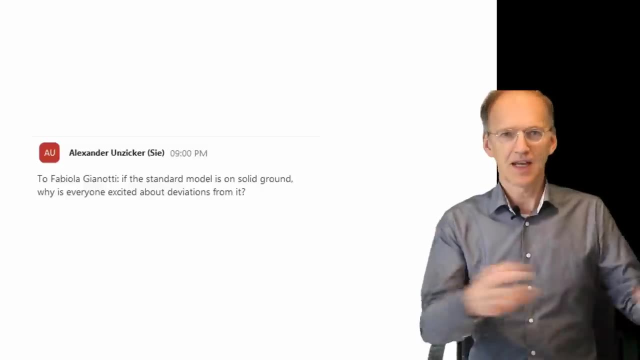 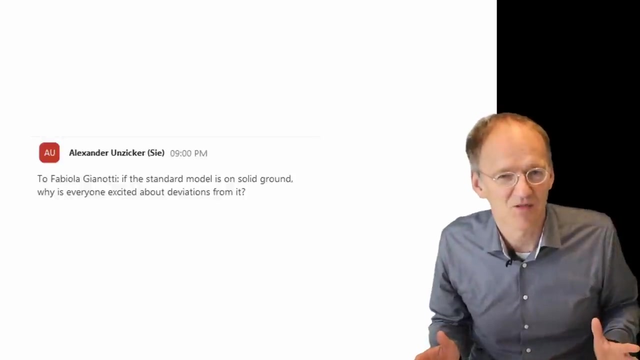 on the one hand side. on the other side It's incomplete. we need to go beyond. we need to explain dark matter, we need extensions. we are excited if something else that contradicts the standard model is discovered. So what do you want at the very? 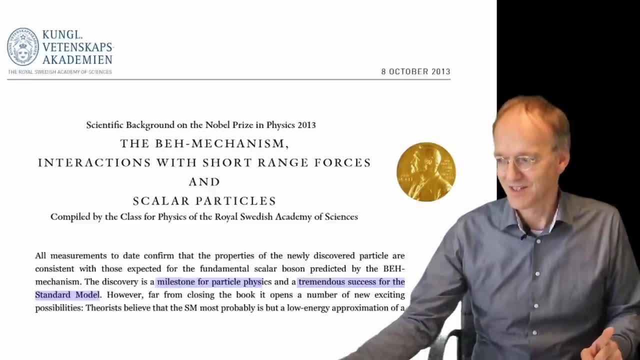 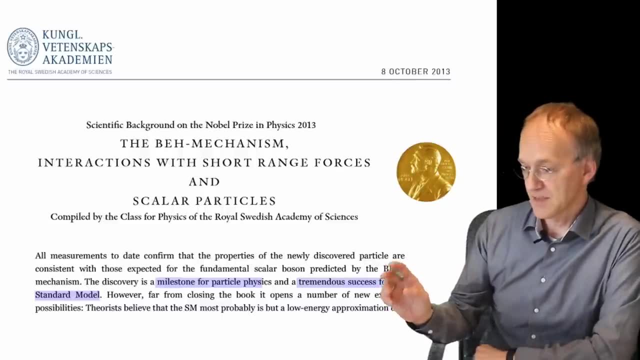 end. I mean this is particularly interesting in the context of the two Nobel prizes in 2013 and 2015.. Look at this: this is the official statement of the Nobel committee and you have the discovery of the Higgs bosons. 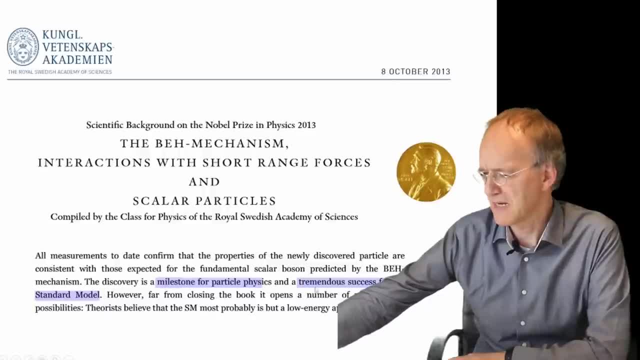 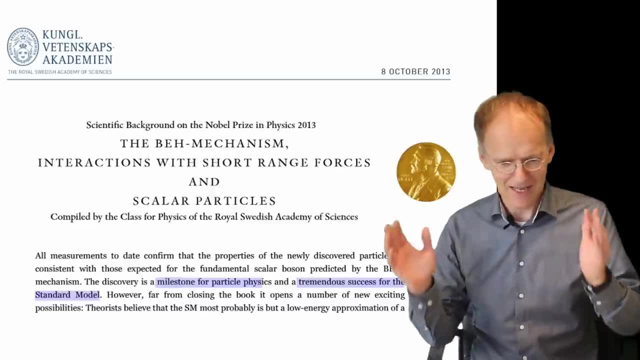 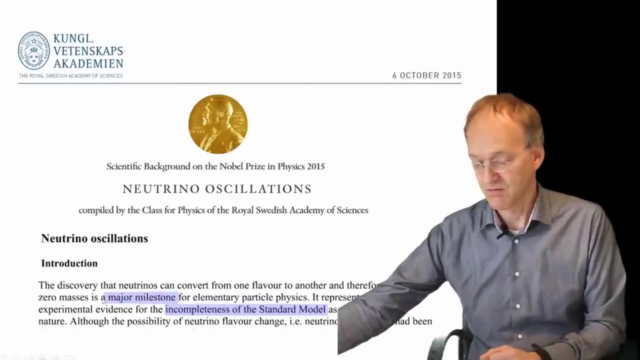 this discovery is a milestone for particle physics and a tremendous success for the standard model, because it ultimately confirmed the standard model and it's validity and we can believe in it. okay, And then, two years later, between your oscillation contradicting the standard model, 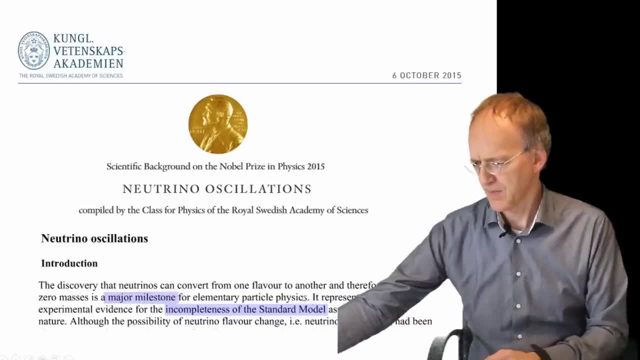 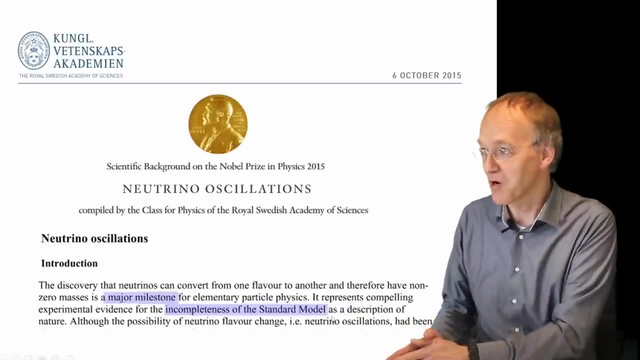 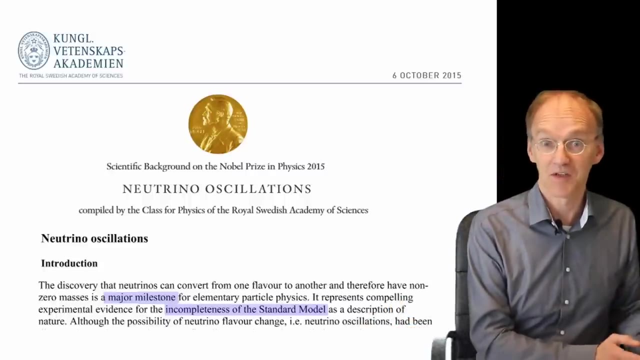 is a major milestone for elementary particle physics. It represents compelling evidence for the incompleteness of the standard model and means that the standard model is wrong 2015.. You get a Nobel for it because it's wrong 2013.. You get a Nobel because it's so fantastic. 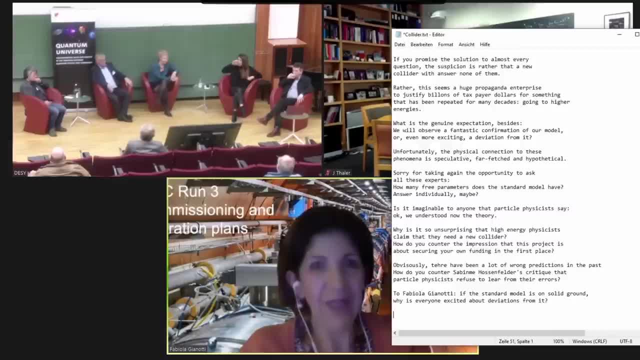 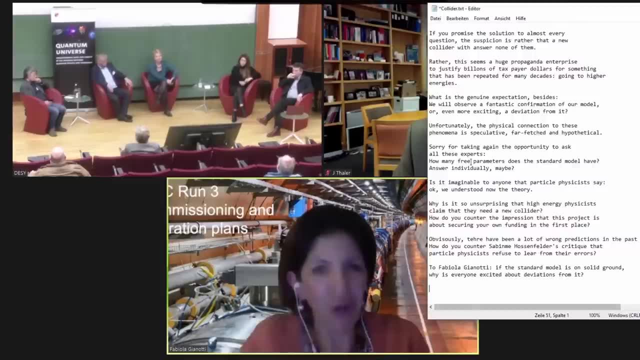 I just don't get this. There are many pieces that are missing, and so we are trying to make the next step and look for the theory, a more general theory, of which the standard model is just a part that can explain everything possibly. 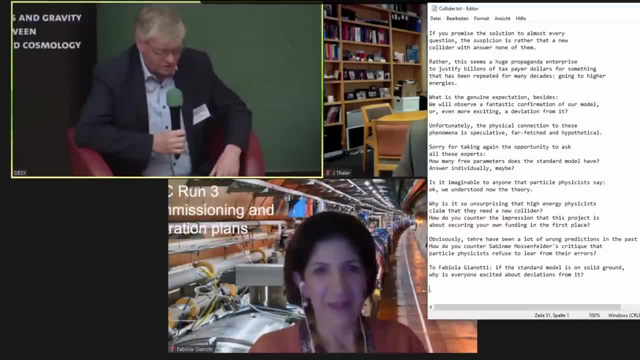 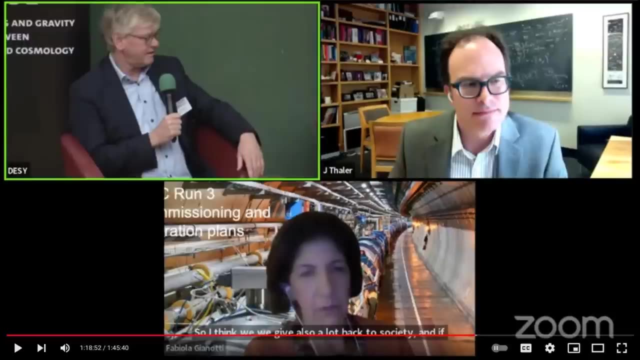 For the scientist who does fundamental research that is confronted with the fact that if you look to the energy density of the universe, that you are able to explain 5% And the rest is dark. I think that's reason enough If the dark matter happens to be in this energy range. 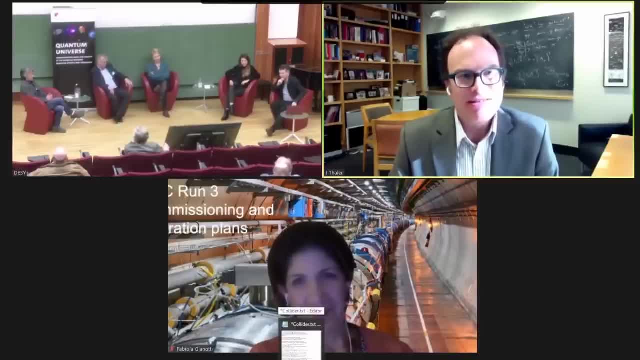 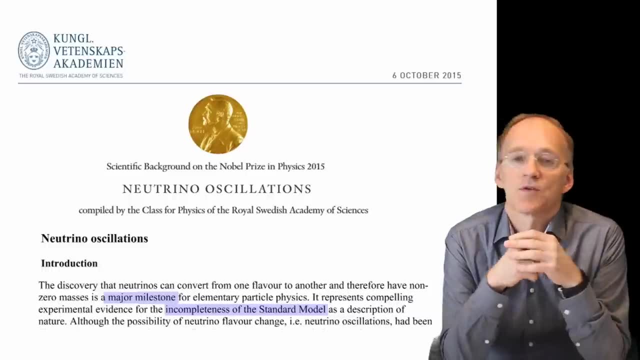 I think that the biggest question- that if we had an answer I could die happy- is: what is the nature of dark matter? And of course, everyone reiterates blah, blah, blah. we need to go beyond. there is dark matter in the universe. I don't understand anything about dark matter. 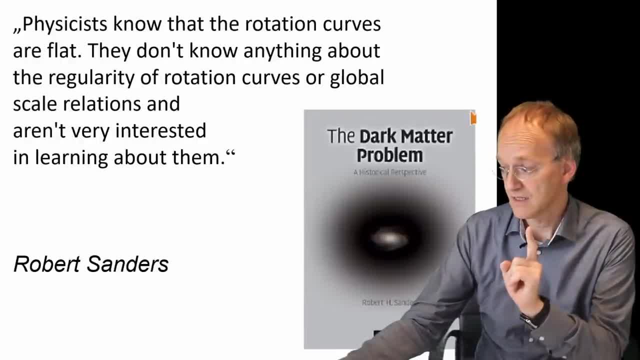 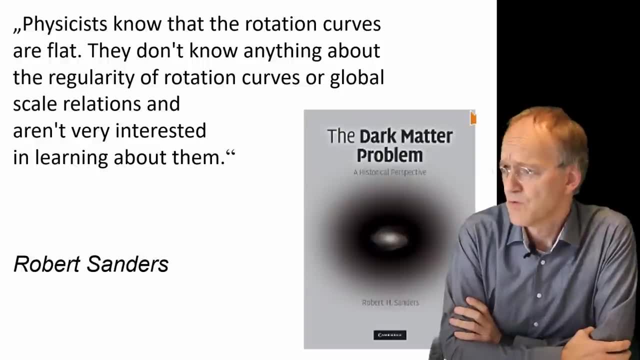 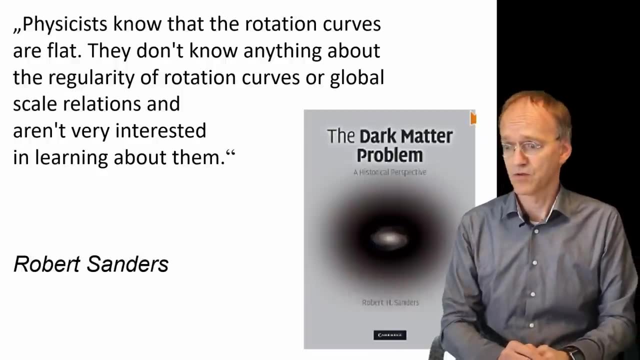 Here is a good point. Someone who really understands something about dark matter says the following: Robert Sanders in his book The Dark Matter Problem. physicists know that the rotation curves of galaxies are flat. They don't know anything about the regularity of rotation curves or global scale relations. 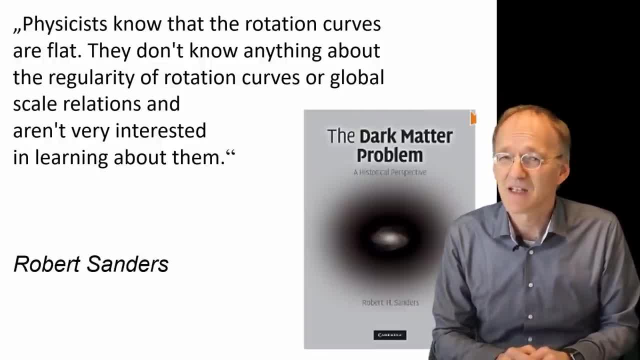 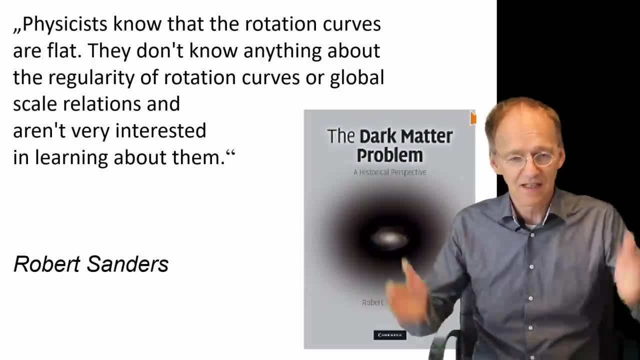 and aren't very interested in learning about them. If you really understand something about galaxy dynamics as Sanders does, you're not going to solve this problem with a single invented particle. Okay, you may hope for 3 or 4 or 5 particles. 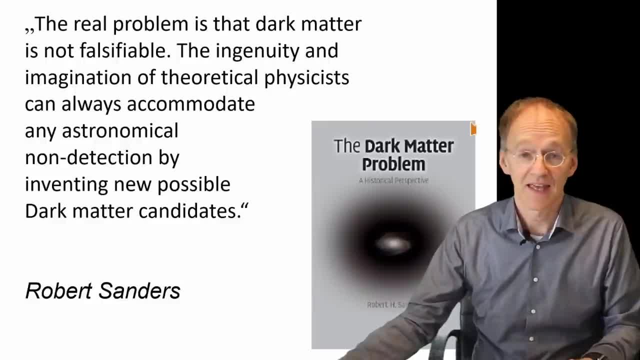 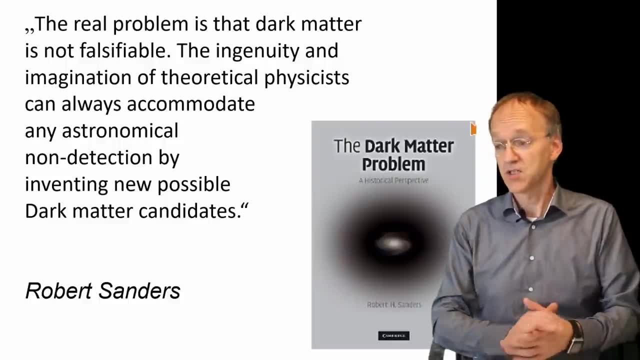 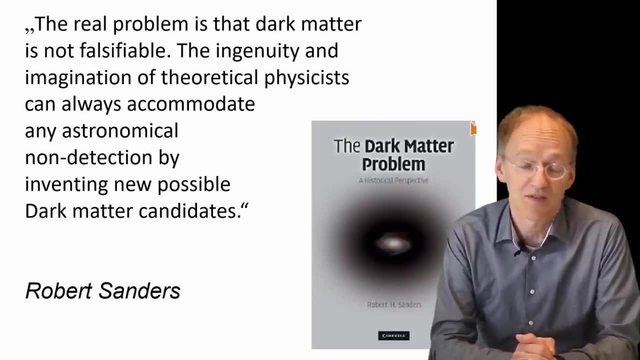 but this is even a bigger mess. And then Sanders says: the real problem is that dark matter is not falsifiable. The ingenuity and imagination of theoretical physicists can always accommodate any astronomical non-detection by inventing new possible dark matter candidates. It is just sufficient you. 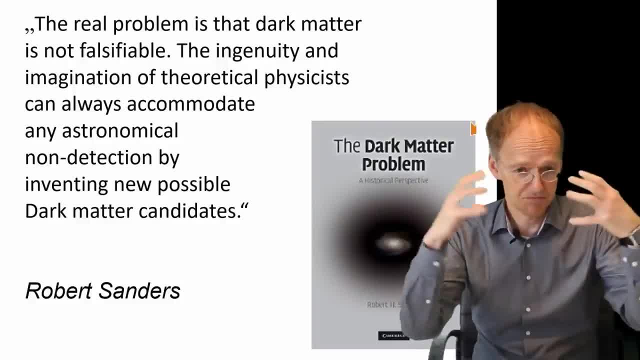 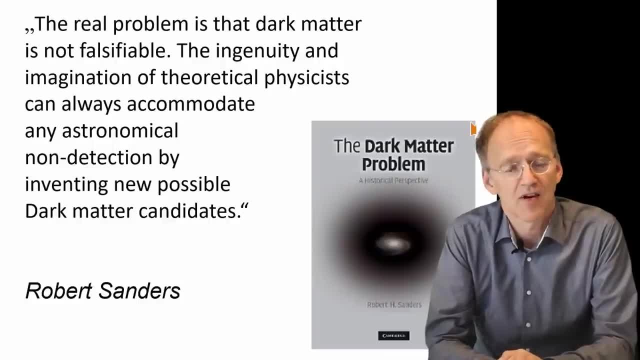 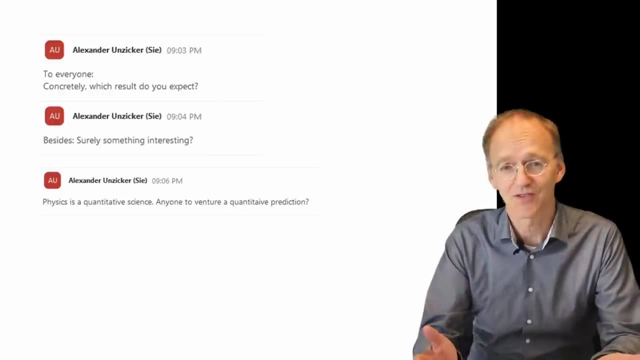 invent some candidate particle, and then you demand a new collider and we must build it and we must look for it. But this is a nonsensical, never-ending hamster wheel. At a certain point I realized I was practically the only one asking questions, so of course I took the opportunity. 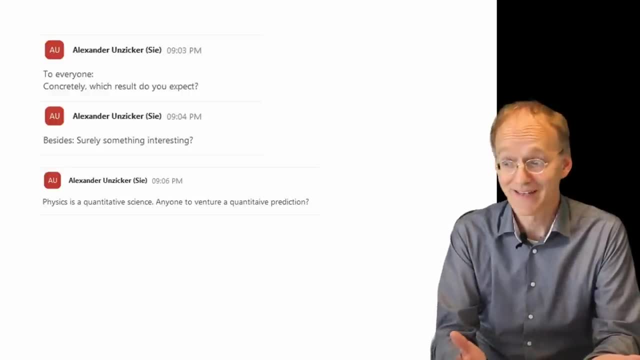 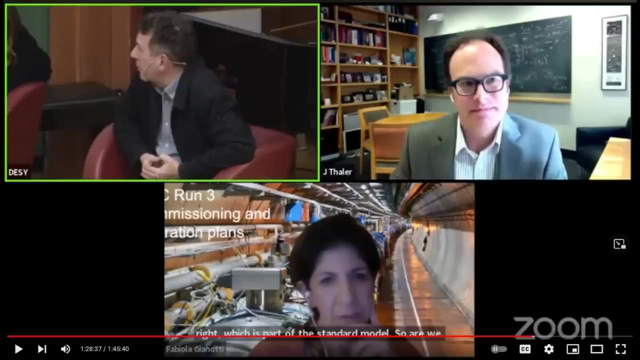 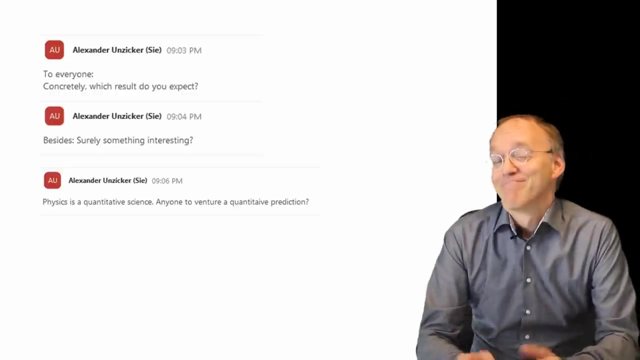 and asked another one to everyone. concretely: which result do you expect besides surely something interesting? What do you hope it will really reveal and what do you think it will reveal? But Butterworth took only the first part, so the answers were: surely something interesting. 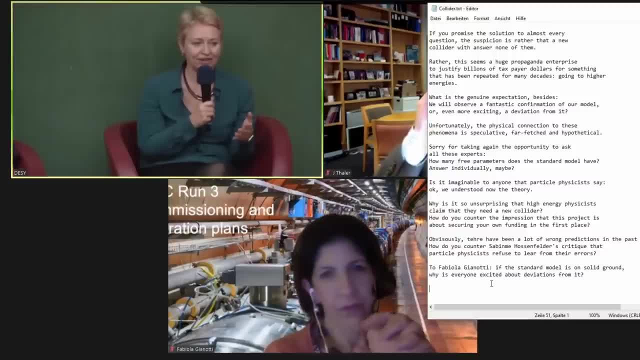 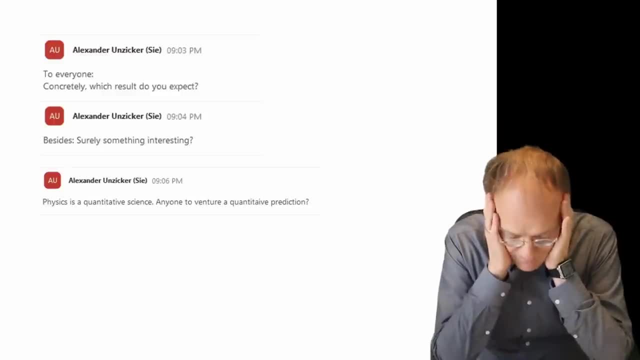 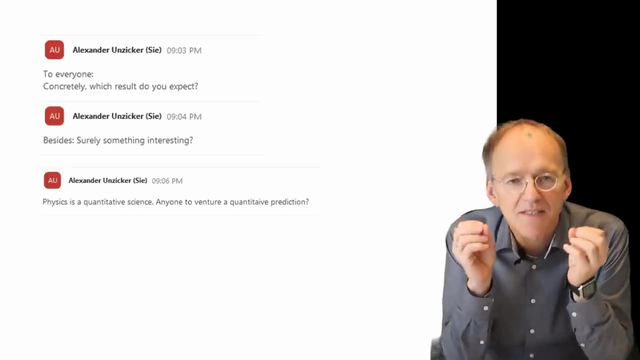 Listen, At the time when Einstein did his work on general relativity, I mean everybody was very happy with Newtonian mechanics, right? How can you compare Einstein's theoretical struggle to understand the basic quantitative anomaly with this messing around with the standard model without no theoretical idea? 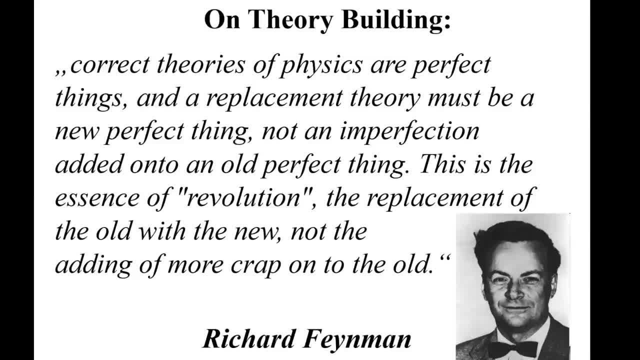 just playing with higher energies. One should add a comment of Richard Feynman here on theory building. Correct theories of physics are perfect things and a replacement theory must be a new perfect thing, not an imperfection added onto an old perfect thing. This is the essence of revolution. 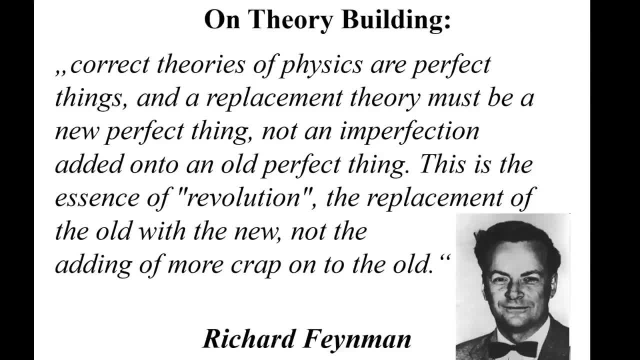 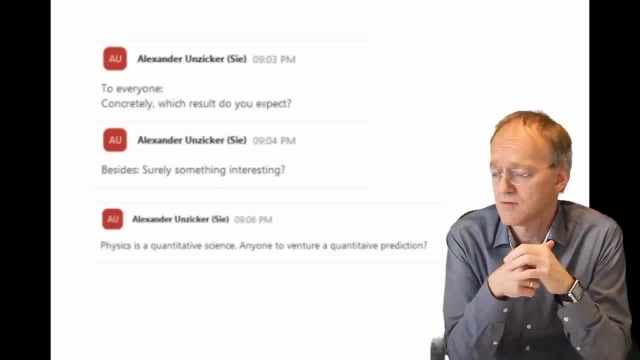 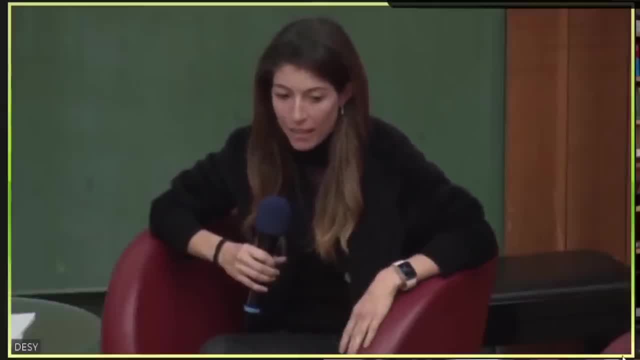 adding more crap onto the old. and this is exactly what the standard model does: adding more crap onto the old. Let's also listen what the others have to say. Another answer: She's cute. I'll try to add a bit, maybe from the experimental side. 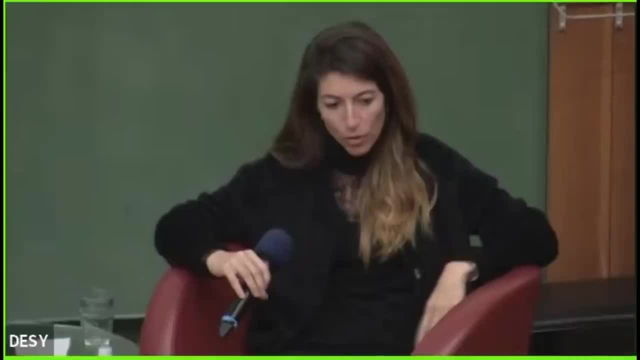 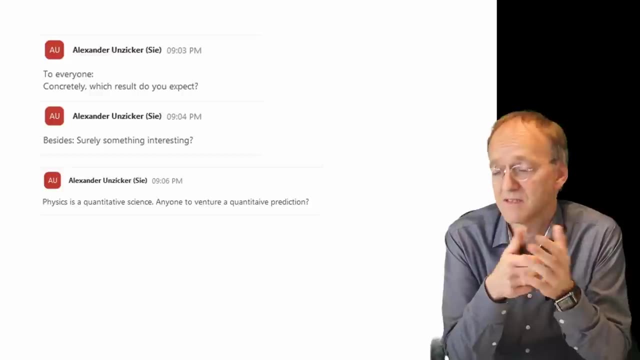 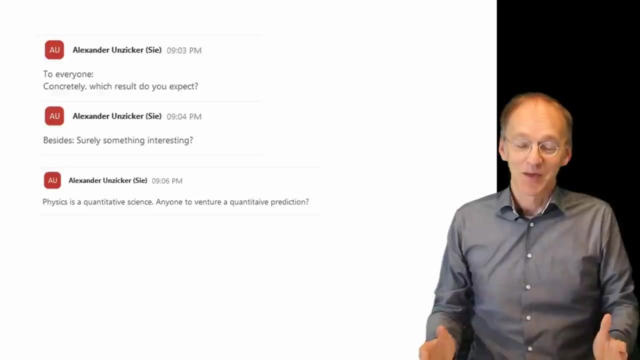 as you mentioned, in the future, we continue to run for more than a decade and we'll have much more statistics. Statistics is interesting. Then I added that physics is a quantitative science and you should make quantitative predictions, and it was a little bit late, I admit, and, of course, 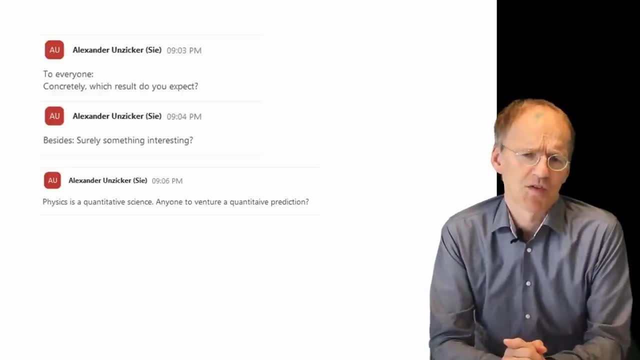 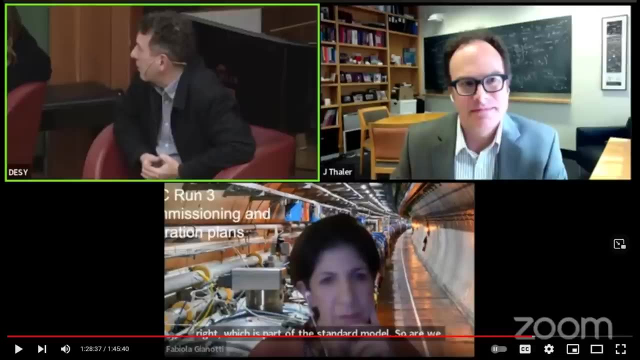 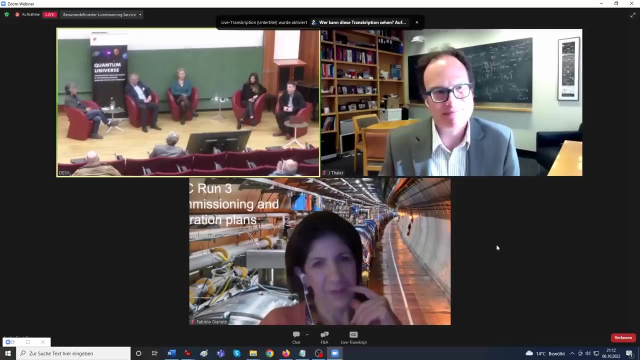 nobody would come out with a number, but it was explained and of course there are numbers behind. That was the last question. I think we should do that. There was one that came in while you were all talking. Physics is a quantitative science and it's not going to give a number on anything. 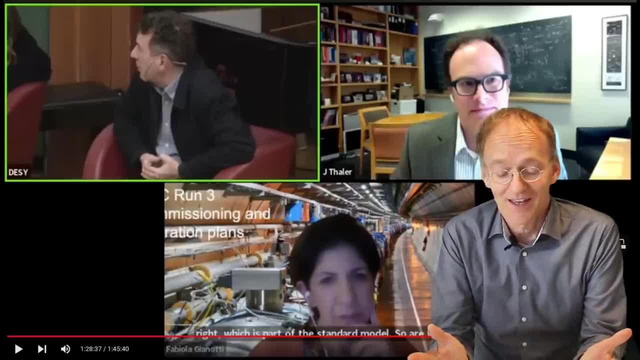 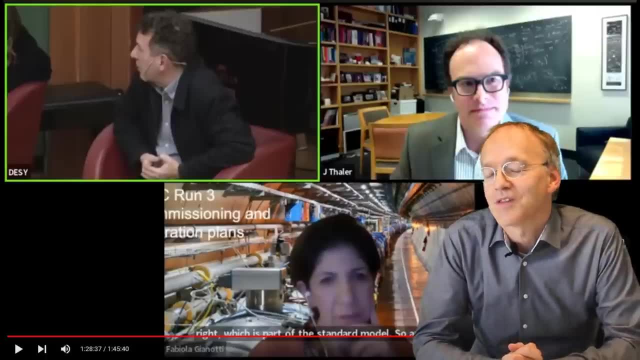 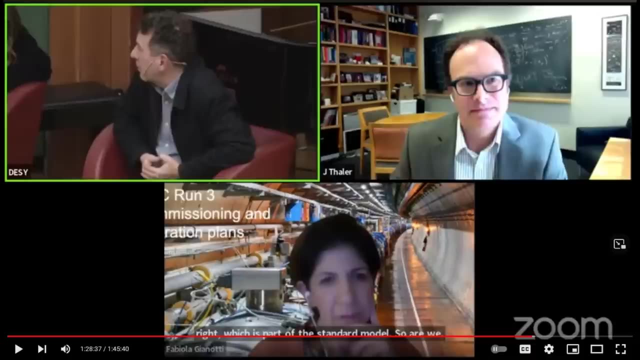 There are numbers behind One question. unfortunately I forgot and I would really like to ask this question: Which result would falsify the standard model? I don't think there is a good answer to that. Time ago I had an argument with a particle physicist who said that she was so excited. 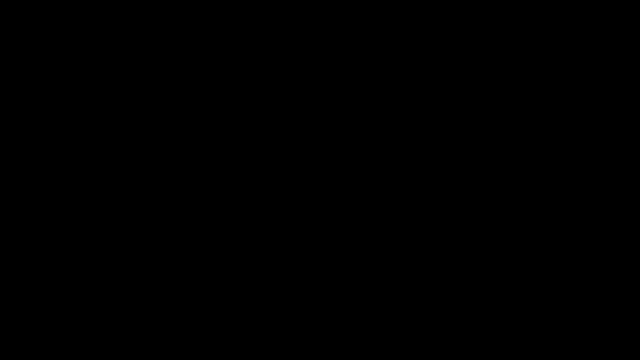 to find new anomalies in the standard model. First thing, I don't believe that you really create the anomalies. These are all buried in some tension that will probably soon drop out, but there is no really tension or really problem created. I don't think that the standard model is falsifiable. 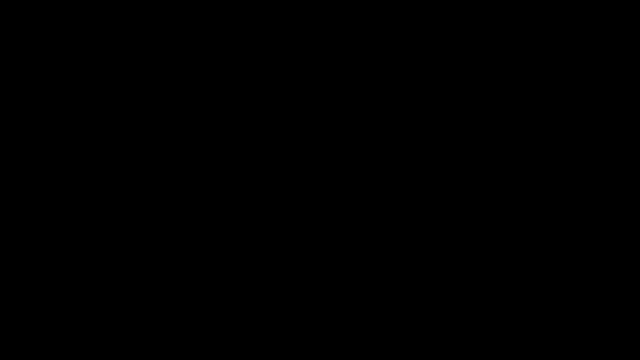 There is no result that could not be digested by some neat extension. This is the first thing, and the second thing is: if you are happy working on the epicycles, let it be, it's ok, That's how scientists are. Thank you, Anyway. So this question and answer session finished. 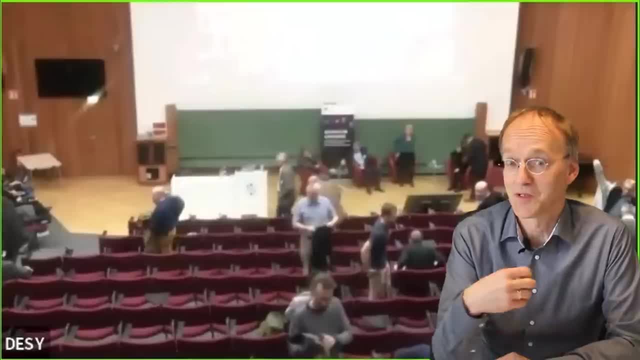 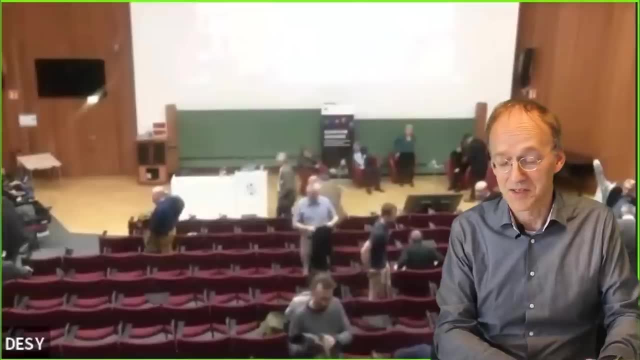 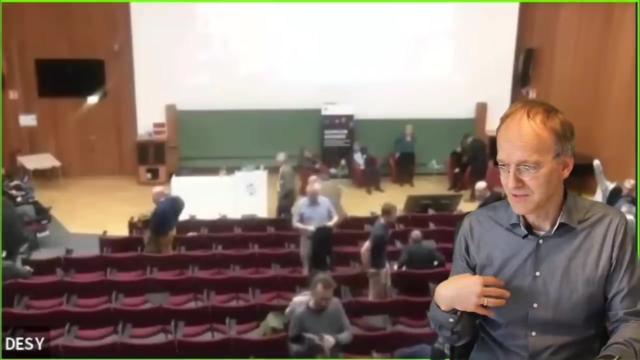 and, yeah, as I said, I was the only person interested in the results of particle physics, obviously in this talk. and then, if you look at the participants, we have here something like 95 online participants and if you look at this picture, I counted 25 in the lecture hall.